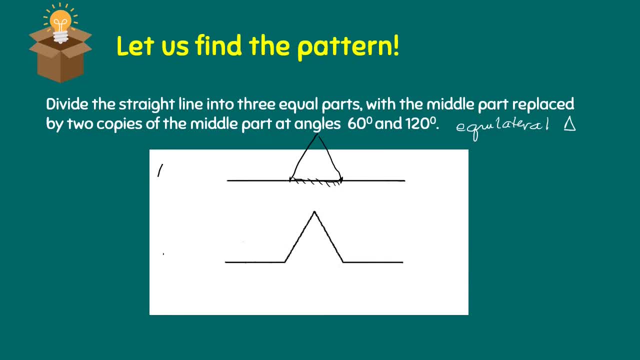 We have how many lines like this we have one times For correct. Okay, so that's the number of segments. and what about the Length? let us assume that. so this is the number of Segments and then this is the perimeter, or anyway, that's just. 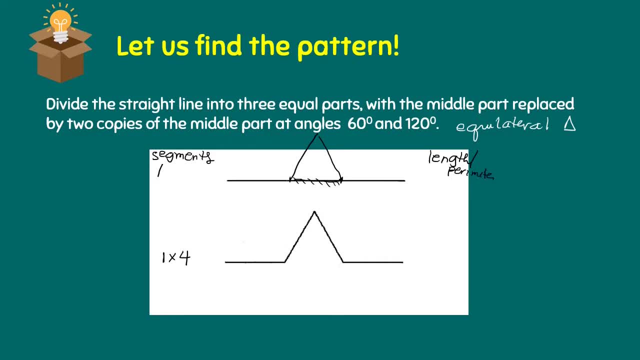 Yeah, probably, just Anyway. so, Assuming that this one Side length of one, since we divide everything we divided equally into three parts, That's one third. Everything has a length of one third, Right? So meaning to say this one, here we have four segments, each of size one third, so the length is 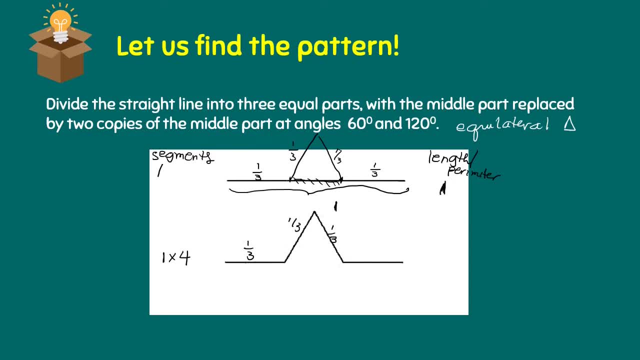 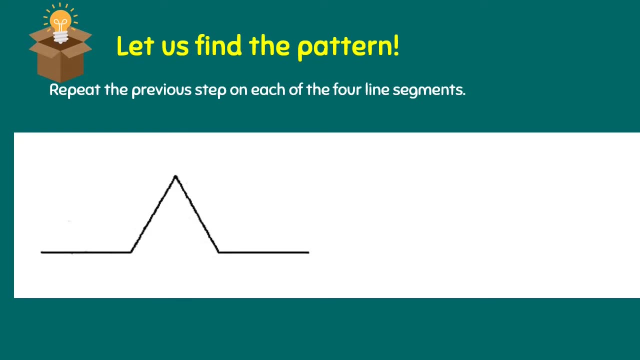 So here the left original length is one, here It's now one third times four, or equal four thirds. Let's look at the next one. So again we repeat the same process. We divide this into three. Okay, divide that into three. Divide that into three, Don't forget we will erase half. 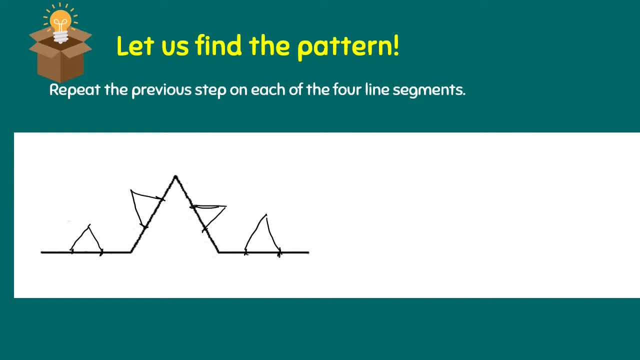 Okay, meaning to say, if we clear that up, Make it cleaner, we will obtain This figure. now, how many segments do we have in our original figure? in our original figure, we have four segments, right segments for nine segments, and We have, we have. we have four segments, but then each. 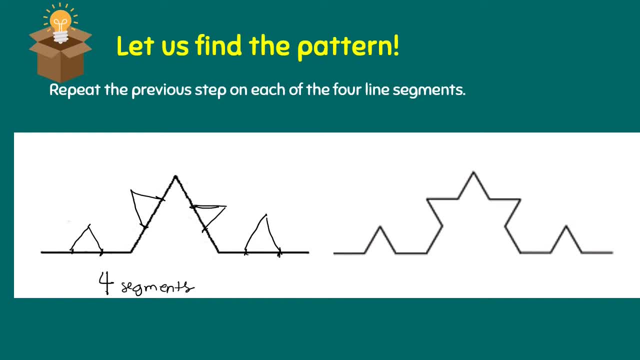 one, two, three, for each of those four segments will turn. it will turn into Four smaller segments, right? So how many segments do we have Now? we have four times four segments. here You have 16 Segments, correct? because this part one segment. it became one, two, three and four. 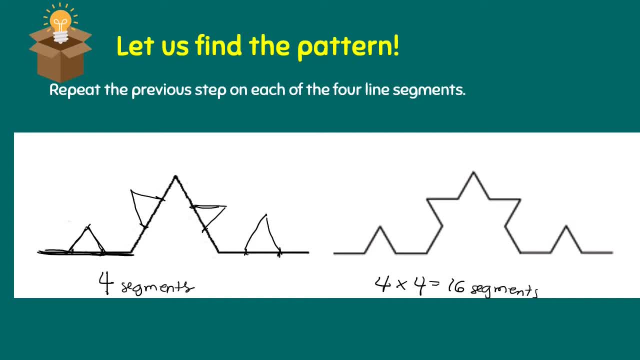 segments. okay, now, what about the perimeter? now, take note that in our previous discussion, this one has a length, has a perimeter of the original, it has a perimeter of four times one third, or four thirds, meaning to say, this one has a length of one third, but in this case, this is now. 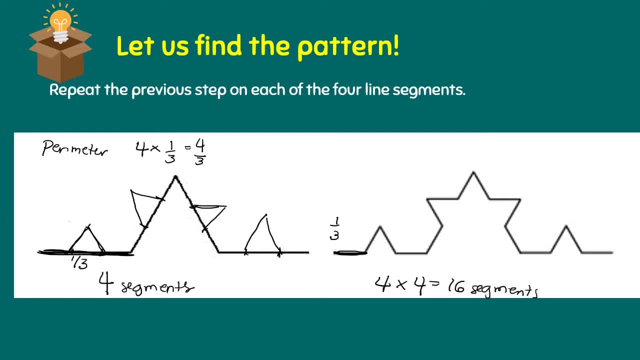 one third divided by three, again right, or one third of one third, or one over nine. so the 16 segments so we have. the perimeter here is four squared times one over three squared, correct? this is the number of segments, this is the length of each segments. okay, so that's four thirds raised to two. so that's 16 over nine, if you repeat. 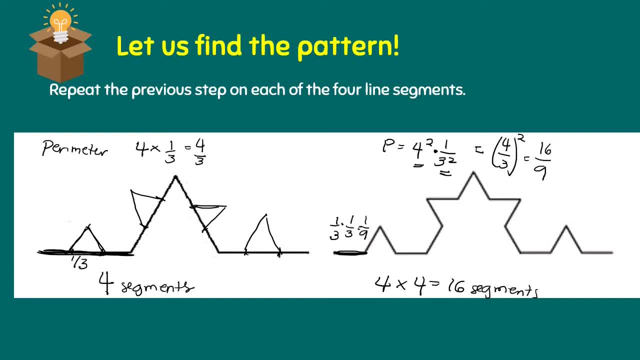 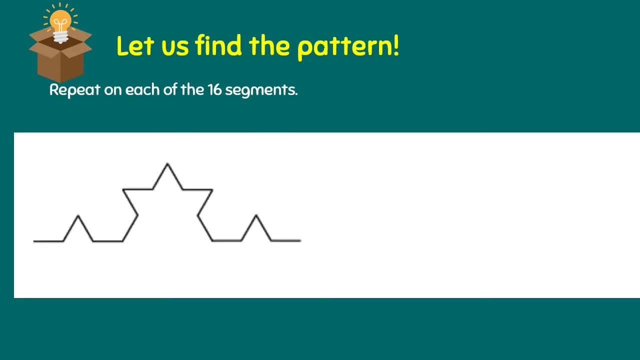 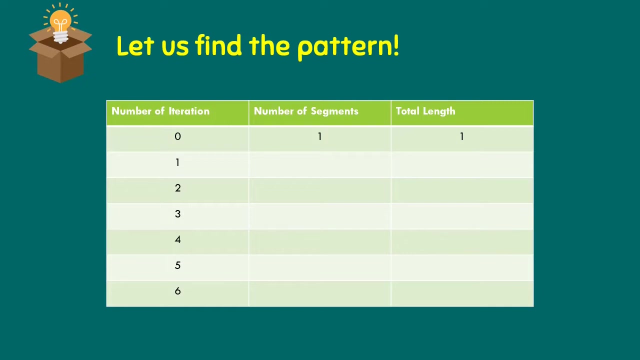 this process again, what do you think is the number of segments and the perimeter? okay, so if you repeat that, okay. so let's summarize what we have seen so far. so if we have, for the first item, for the first, we started with one segment and then we have a total length of one unit, and then, if we have on 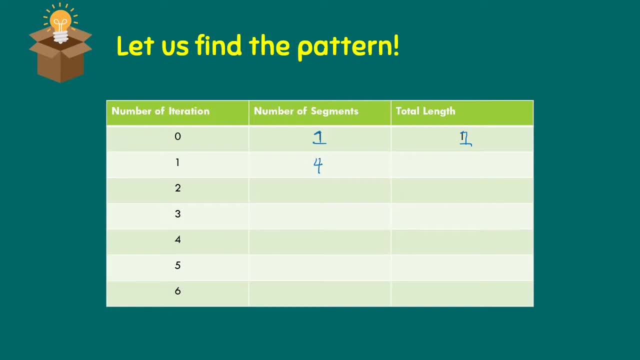 the first iteration. so we already have four segments and the total length of four, over three seconds. and then on the second iteration, those four segments, each of those um segments, turned into four smaller segments. so we now have four times four, so four squared, and a total length of 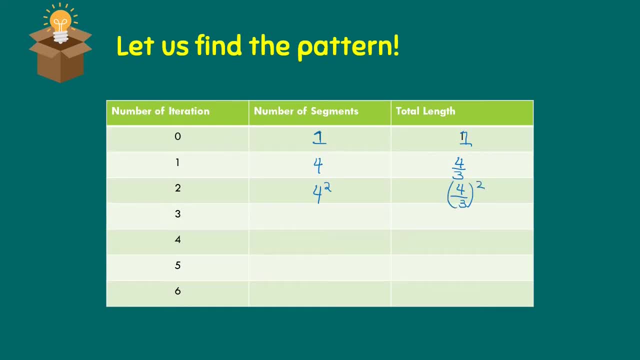 four thirds squared. so can you now guess what will be the number of segments on the third iteration? it's four cube, this is four thirds cube, and so on. so therefore, the number of segments on the third, let's just make this in so if we have, for the end iteration, the total number of segments that we 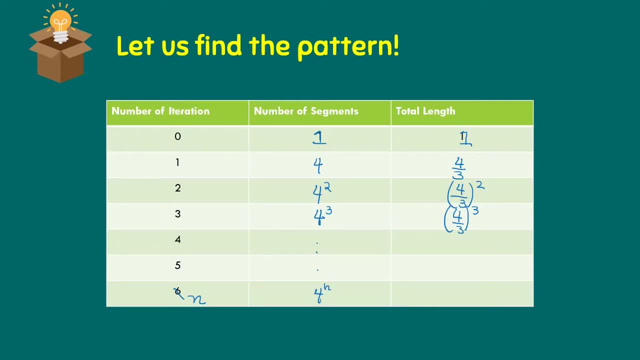 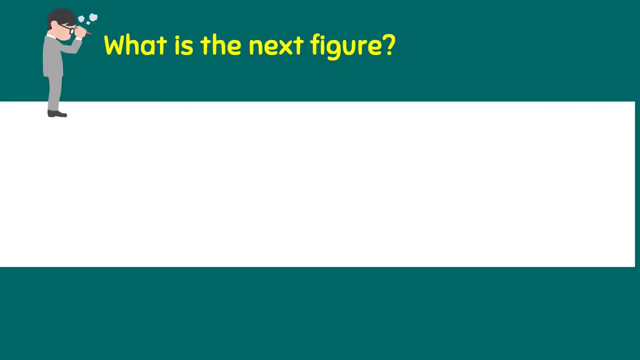 have is four raised to the end and a total length of four thirds raised to n. so, as you can see, as we increase the number of iterations, the total length of our um figure increases, and okay, so this is the cook edge. okay, let's now look at the next figure. we have here a triangle. 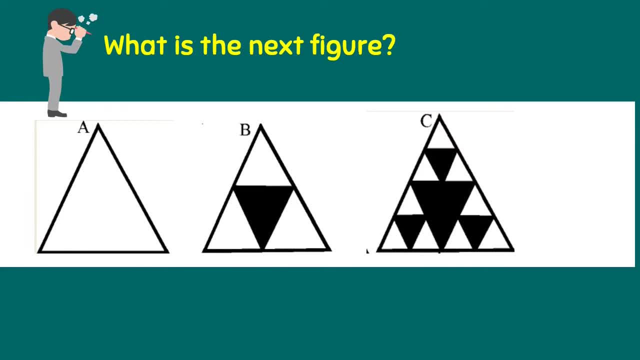 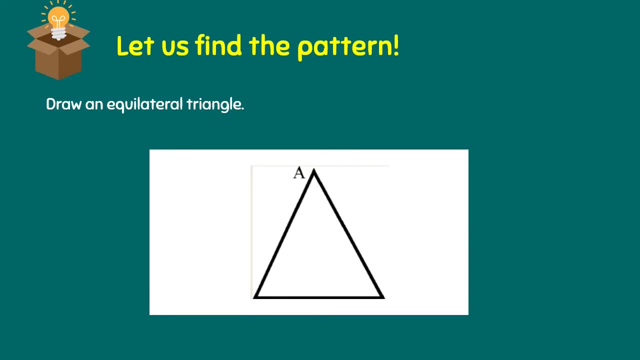 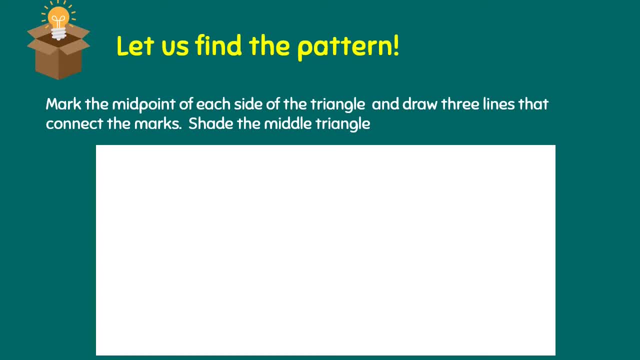 triangle. we mark the midpoint of each side of the triangle and draw three lines that connect the marks and then we shape that middle triangle. so we have this, and then we get the midpoint, midpoint, midpoint, and connect the three midpoints and then shape the triangle. so therefore we have the second figure. okay. 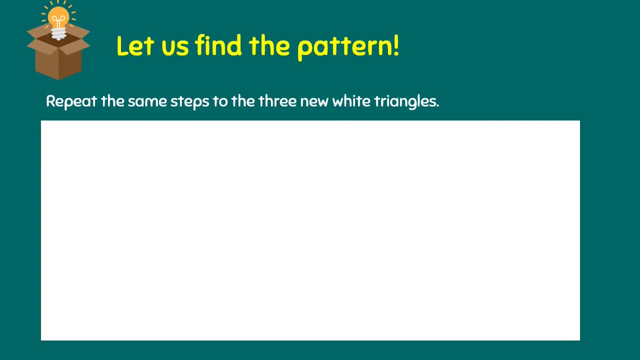 and then we repeat the same steps to the three new white triangles. so remember, we only do those steps for the white triangle. so this figure that we originally had- and then get the midpoint again- midpoint, midpoint, midpoint, connect and then shade, midpoint, midpoint, midpoint, and then shape. okay, so this is the figure that we have. so if we continue to do the same step again, 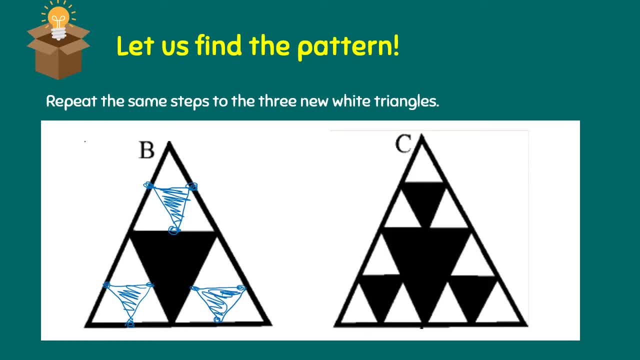 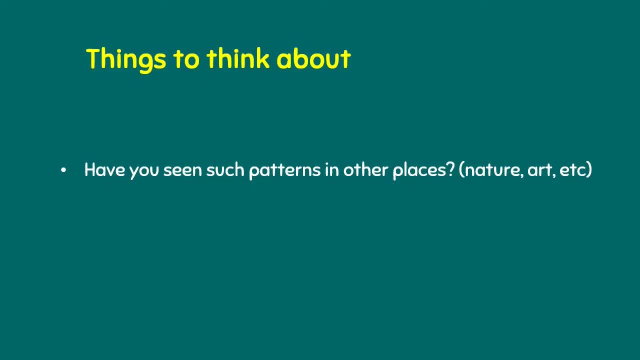 triangle, triangle, that is what we call the Serpinski triangle. Okay, So I seen such patterns in other places: 목ich อ. um, we will see later that. um, these patterns are everywhere, and what is common among the two items that we discussed? uh, basically, what happened is that you always just have to repeat. 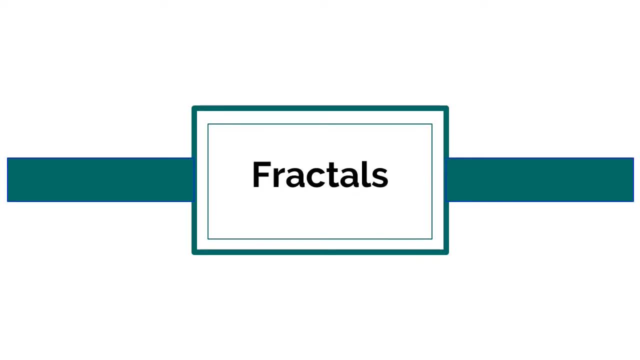 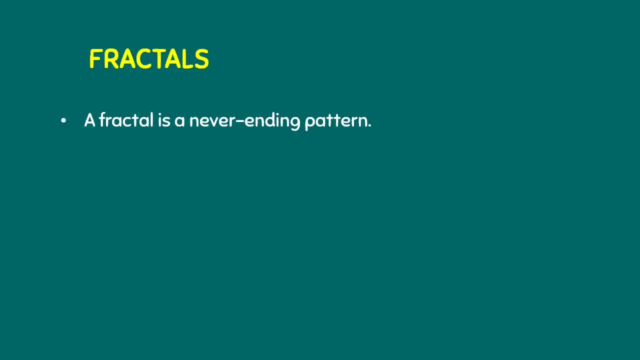 the same process, so the things that we have discussed are what we call fractals. what are fractals? a fractal is a never-ending pattern and they are infinitely complex patterns that are self-similar across different skills. i will talk about this term- self-similar- later in the next. 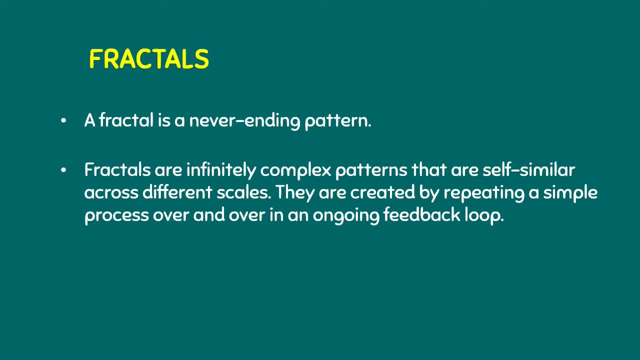 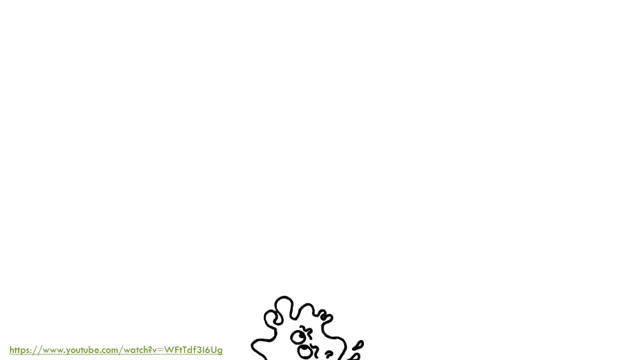 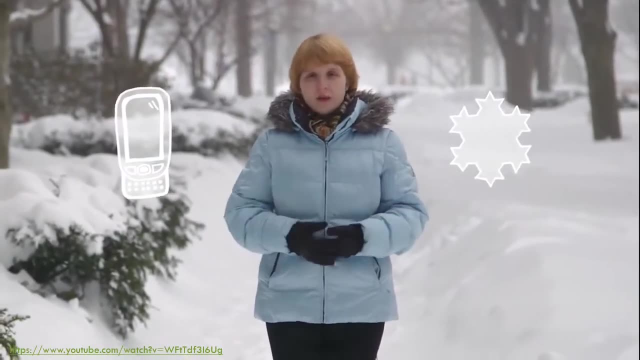 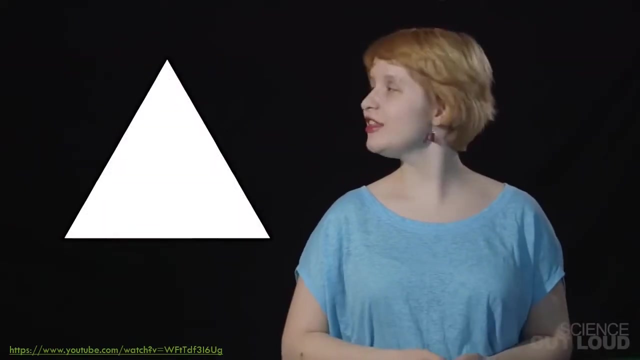 few slides. they are created by repeating a simple process over and over in an ongoing feedback loop. what does snowflakes and cell phones have in common? the answer is: never-ending patterns called fractals. let me draw a snowflake. i'll start with an equilateral triangle. 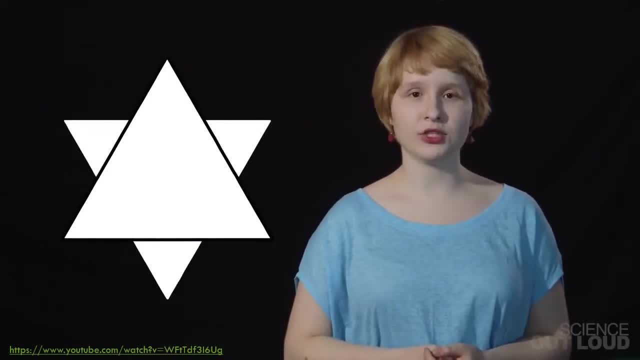 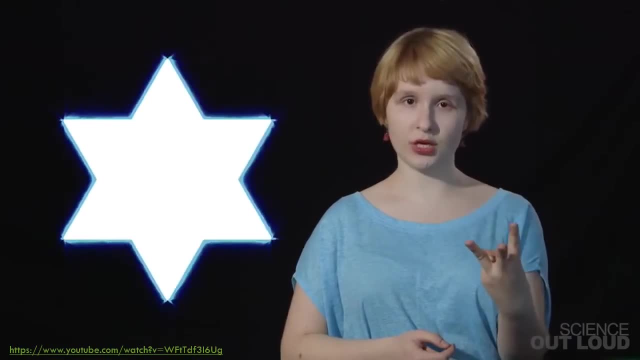 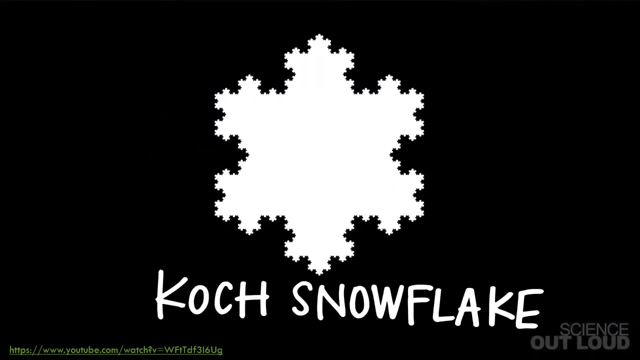 then i'll draw another equilateral triangle on the middle of each side, pull out the middle and repeat the process, this time with one, two, three, four times three, which is 12 sides. if i do this over and over, the shape will look something like this: this is called a coke snowflake and it has. 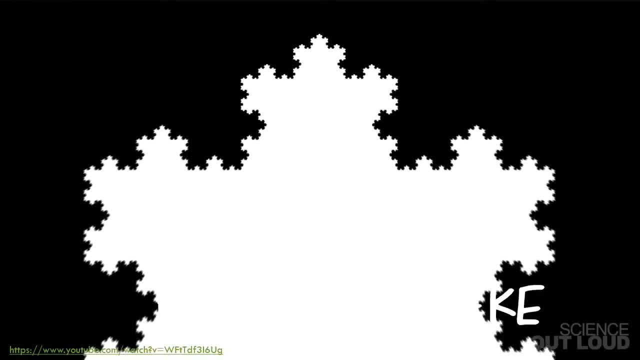 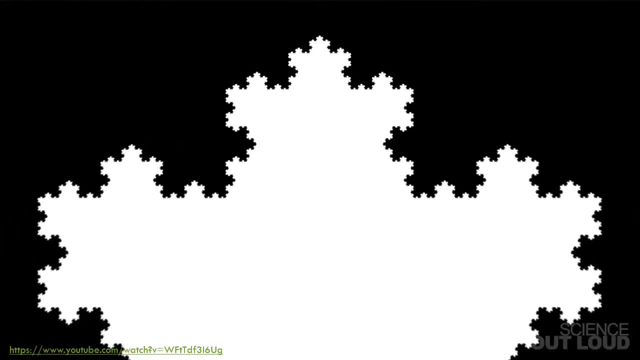 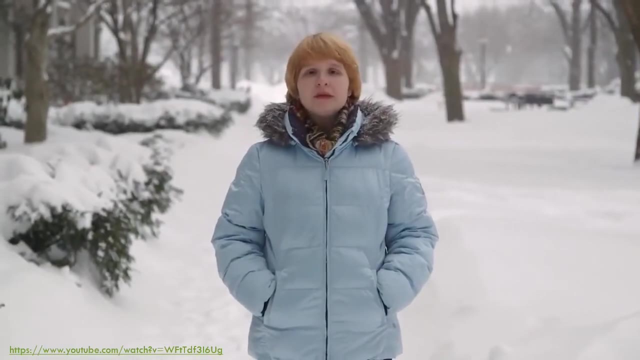 a special property. no matter where i look or how much i zoom in, i will see the same pattern over and over. never-ending patterns like this that, on any scale, on any level of zoom look roughly the same, are called fractals. we can actually draw a coke snowflake on the computer by having it repeatedly. 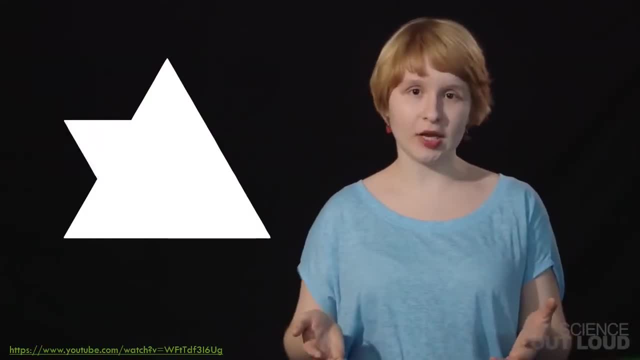 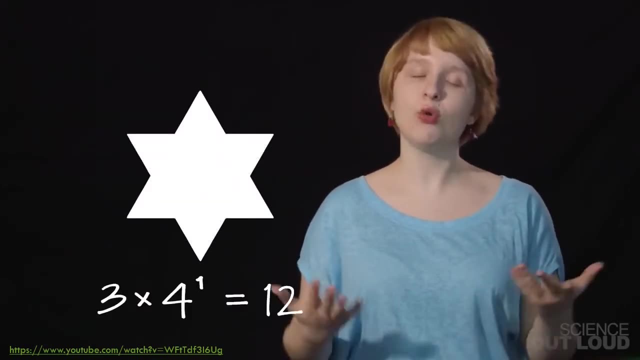 graph a mathematical equation. each time we add a triangle, one side of the coke snowflake will turn into four. after the first repetition, we'll get three times four to the first, or 12 sides. after the second repetition, we'll get three times four to the second, or 48 sides. 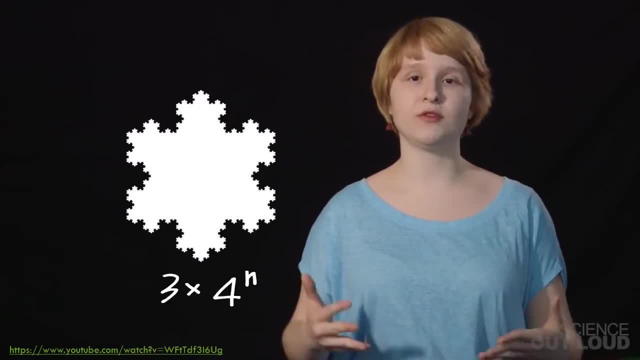 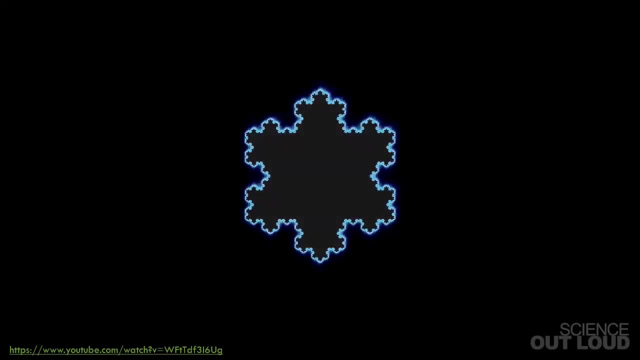 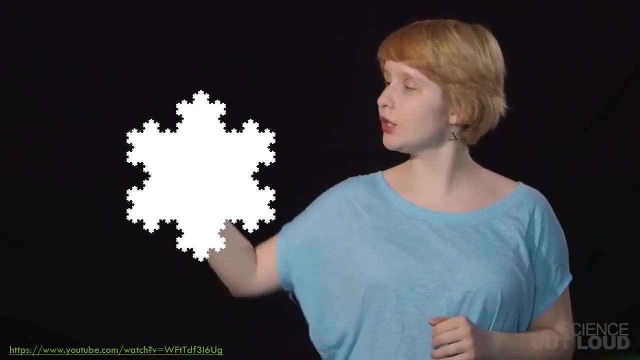 after repetition number n, we'll have three times four to the n sides. if we do this an infinite number of times, we'll get infinitely many sides. so the perimeter of the coke snowflake will be infinite. but the area of the coke snowflake wouldn't be infinite if i draw a circle with. 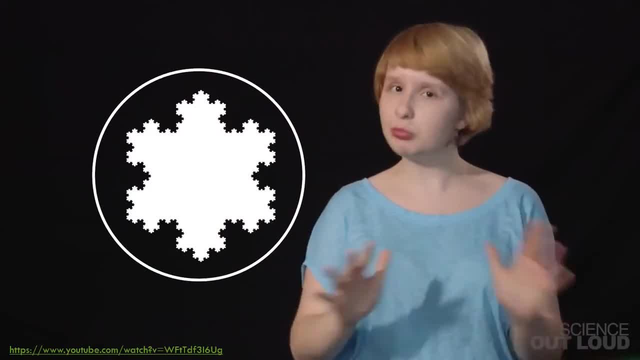 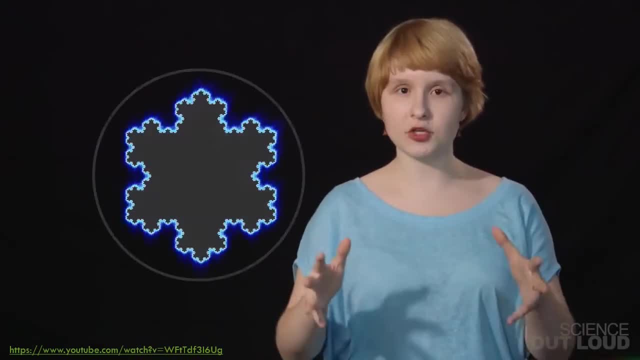 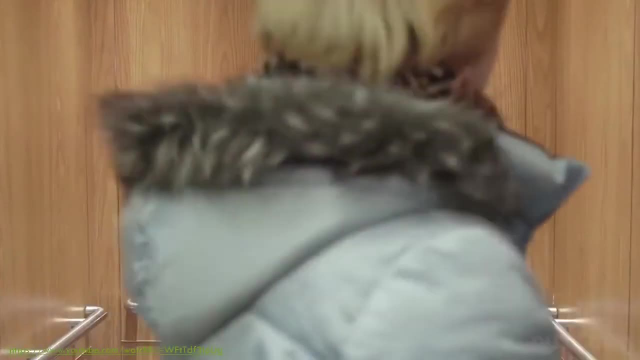 a finite area around the snowflake. it will fit completely inside, no matter how many times we increase the number of sides. so the coke fractal has an infinite perimeter, but a finite area will be infinite. in the 1990s, a radio astronomer named nathan cohen used the fractal antenna to rethink. 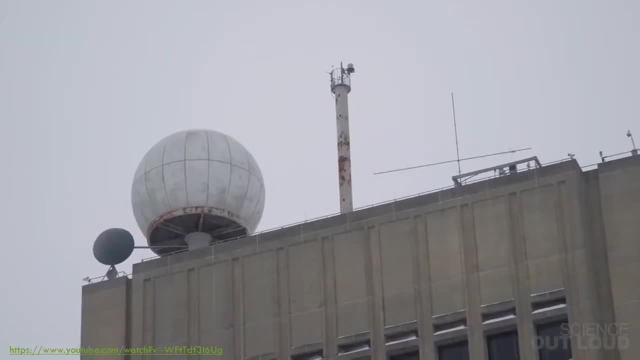 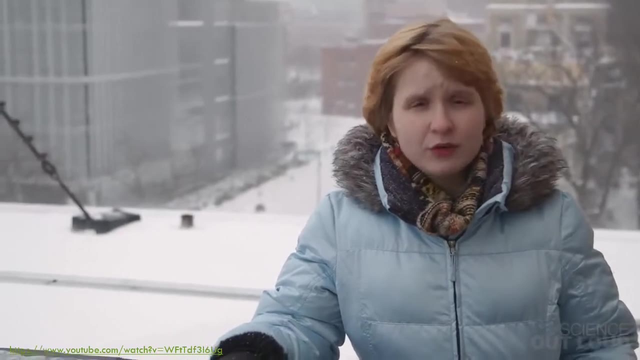 wireless communications. at the time cohen's landlord wouldn't let him put a radio antenna on his roof, so cohen decided to make a more compact fractal-like radio antenna instead. but it didn't just hide the antenna from his landlord, it also seemed to work better than the. regular ones. regular antennas have to be cut for one type of signal and they usually work best when their lengths are certain multiples of their signals wavelengths. so fm radio antennas can only pick up fm radio stations, tv antennas can only pick up tv channels and so on, but fractal. 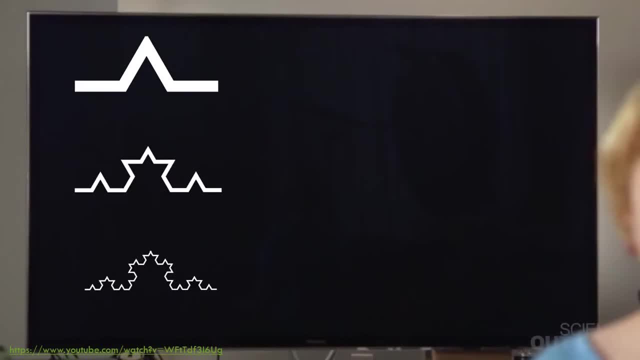 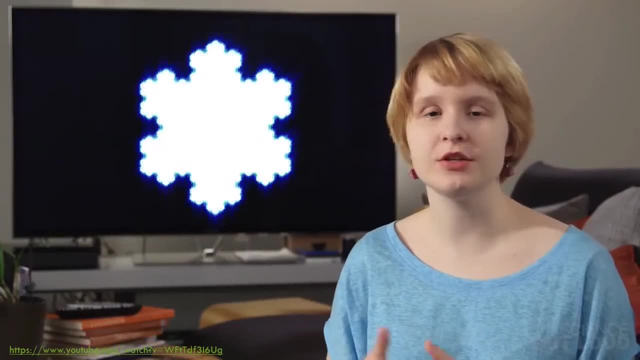 antennas are different. as the fractal repeats itself more and more, the fractal antenna can pick up more and more signals, not just one. and because the perimeter of the coke snowflake grows way faster than its area, the fractal antenna only takes up a quarter of the usual space. 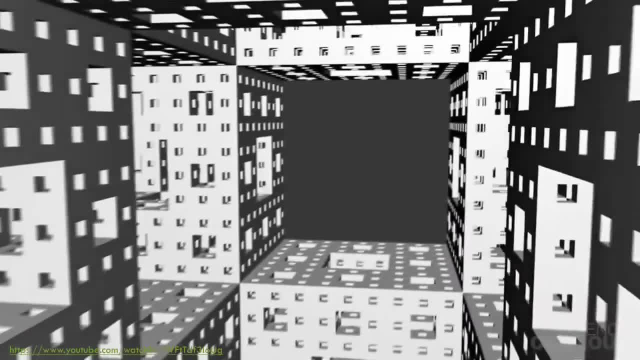 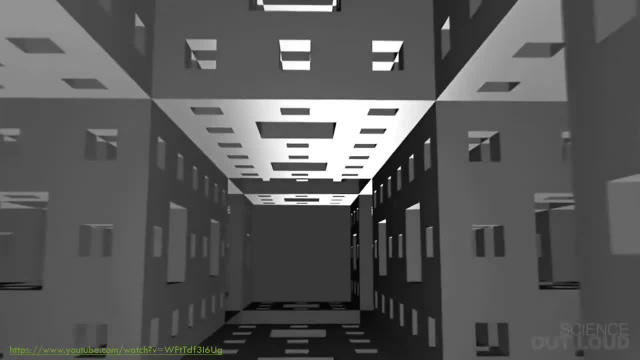 but cohen didn't stop there. he designed a new antenna, this time using a fractal called the menger sponge. the menger sponge is kind of like a 3d version of the coke snowflake: it has infinite surface area but finite volume. the menger sponge is sometimes 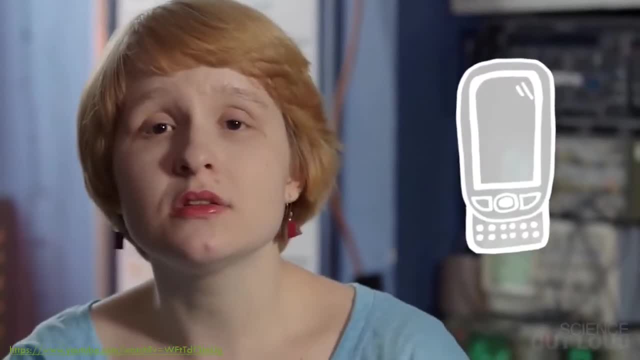 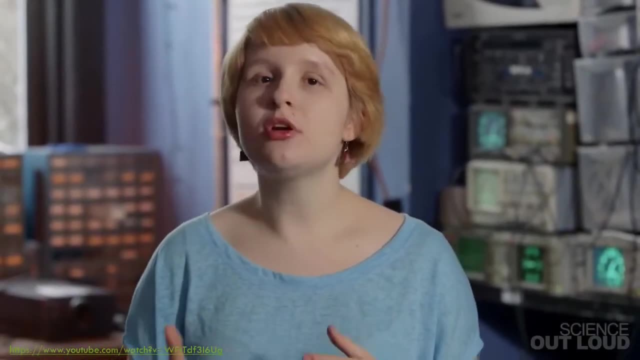 used in cell phone antennas, it can receive all kinds of signals while taking up even less area than a coke snowflake. now, these antennas aren't perfect. they're smaller, but they're also very intricate, so they're harder and more expensive to make. and although fractal antennas can receive, 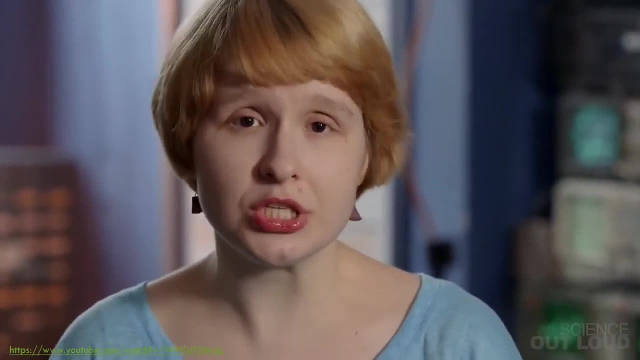 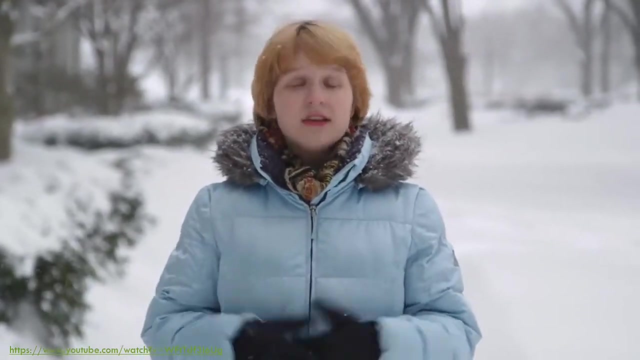 many different types of signals. they can't always receive the same signal. as the coke snowflake, each signal, as well as an antenna that was cut for it. cohen's invention was not the first application of fractals. nature has been doing it forever, and not just with snowflakes. you can see fractals in. 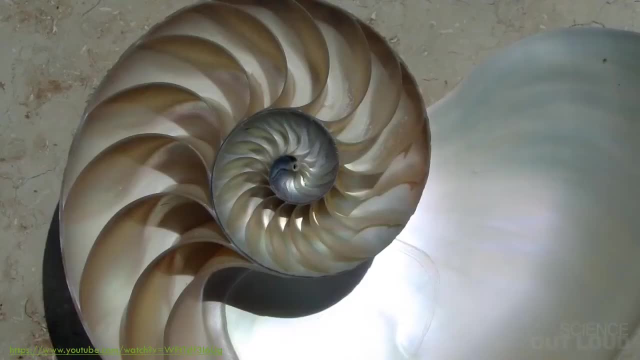 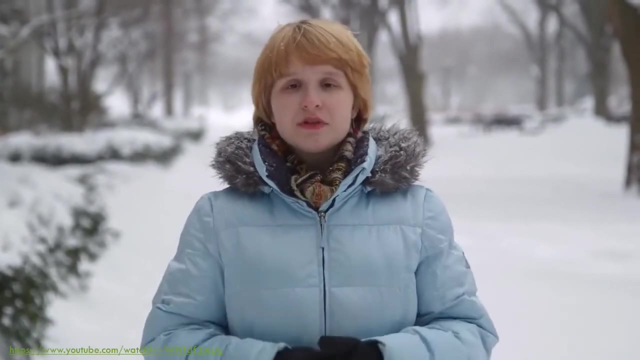 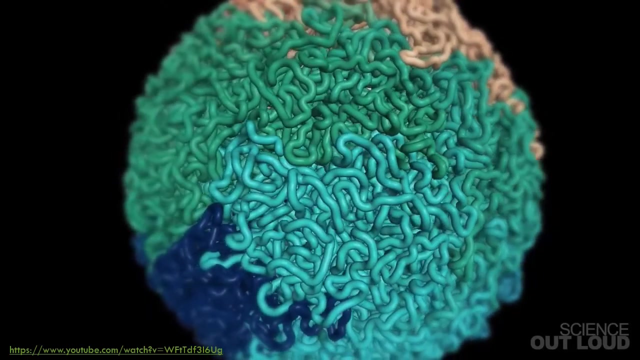 river systems, lightning bolts, seashells and even whole galaxies. so many natural systems previously thought off limits to mathematicians can now be explained in terms of fractals, and by applying nature's best practices we can then solve real world problems. fractal research is one of the most common ways to solve these problems, in the field such as biology, for example, mit. 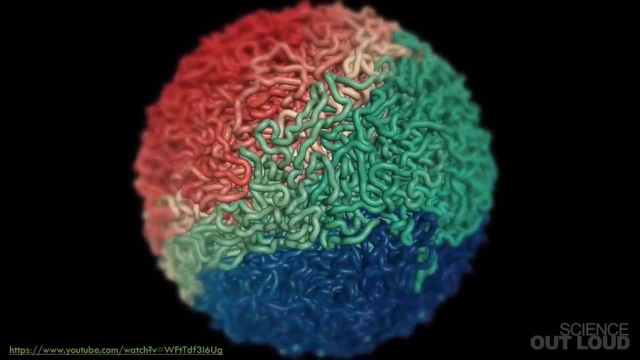 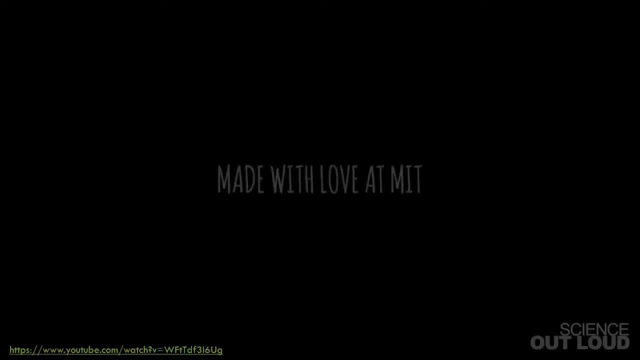 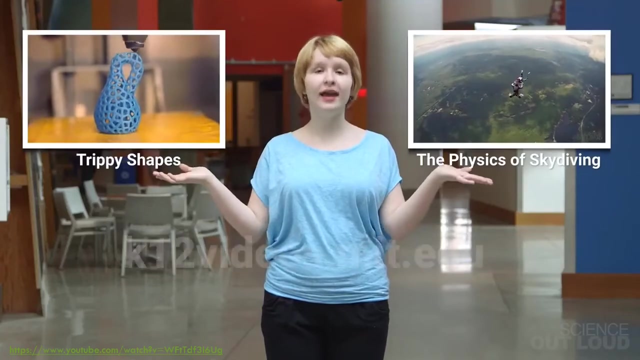 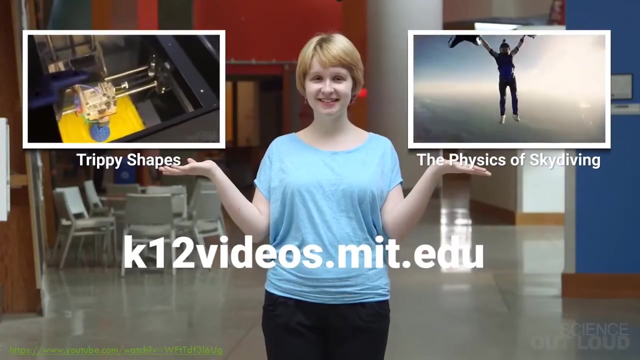 scientists discovered that chromatin is a fractal and that keeps dna from getting tangled. look around you. what beautiful patterns do you see? hi, i'm yulia. thanks for watching science out loud. check out these other awesome videos and visit our website and i'll see you soon. 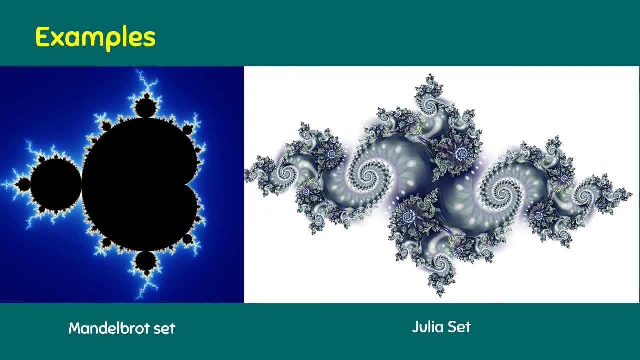 so we're here in the lab. here are some examples of fractals. we have the mandelbrot set, we also have the julia set. so as you can see over here the pattern, if you zoom in, okay, you will again see the same pattern. so there. 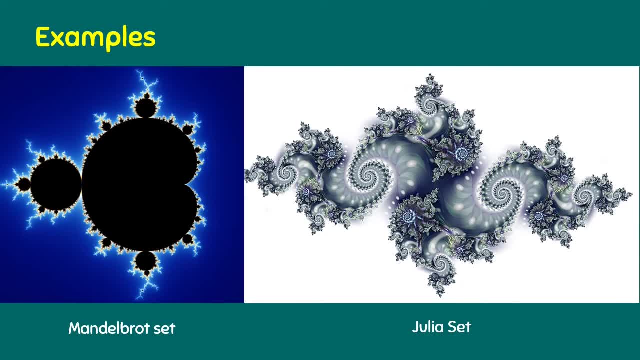 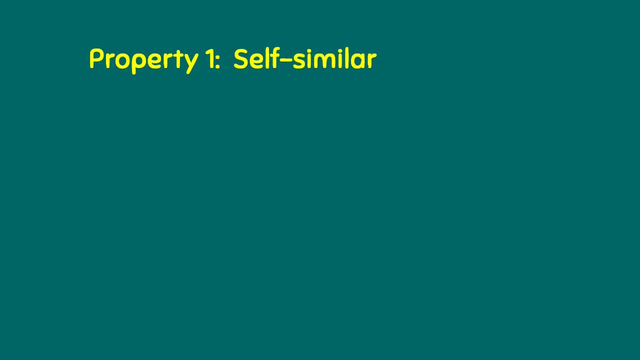 about this mandolin row and the julia set. okay, so let's look at the properties of fractals. the first property that they have is that they are self-similar. so self-similar objects are objects that appear the same under magnification. they are composed of smaller copies of themselves. so for 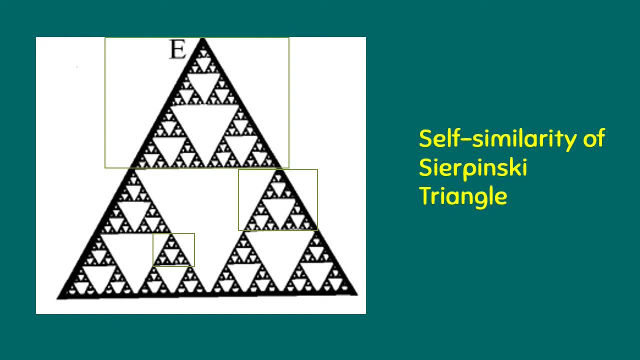 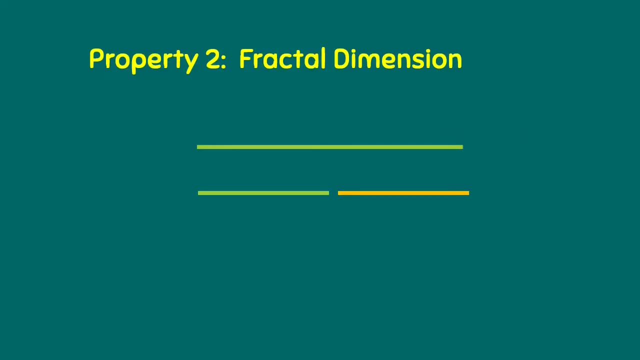 example, if you look at the um serpinski triangle, if you look at this one: okay, this is the small version, this is the bigger version, and then the right, and then, if you continue to zoom in, okay, if you continue to zoom in, you will still see the same pattern. okay. so the second property of 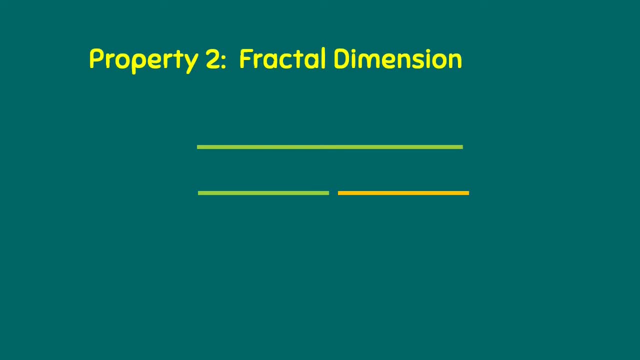 is they have a, a, a, a fraction, as a dimension. what do i mean by that? so first let's look at um, let's start with a one dimensional figure. so i have here a line and then i divided the line into two parts- okay, into two equal parts. so basically they're just the same lines, except that this is a smaller version of. 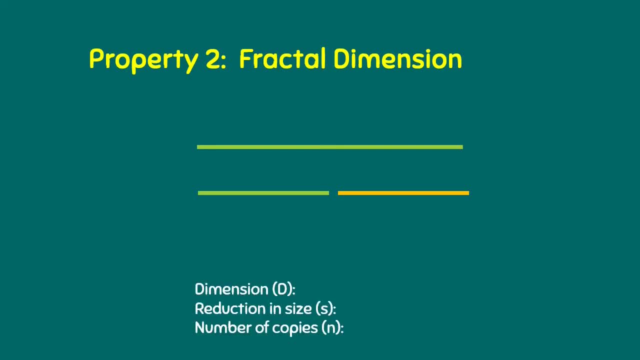 this one. so the dimension, the dimension of our figure, is one: the reduction in size. since we divided the, the line, the original line, into two equal parts, the reduction in size is one half. and then the number of copies rn is equal to 2, because we ended up with two um figures, two smaller figures which 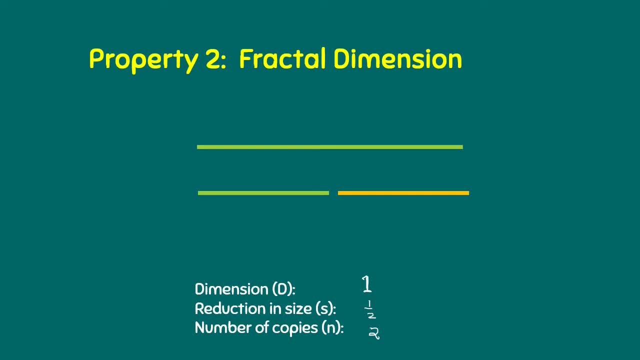 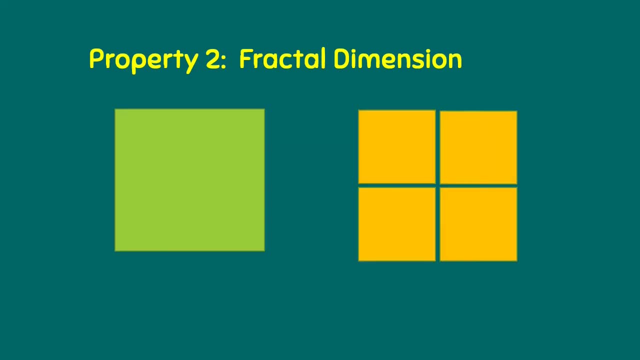 is, which are similar to the original figure. okay, next let's look at this one. so we have here a triangle, and then what we want to do is we want, for each segment, we again get the midpoint. okay, we get the midpoint and then connect the midpoints. therefore, we will end up with 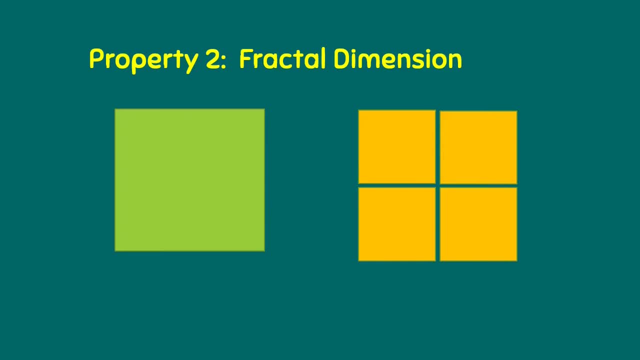 four squares, which are four smaller squares which are similar to the original square. so, in this case, the dimension, what is our dimension? this is two dimensional object because it has a length and width, so two reduction in size, since we divided each of the segments um into two, the segments of 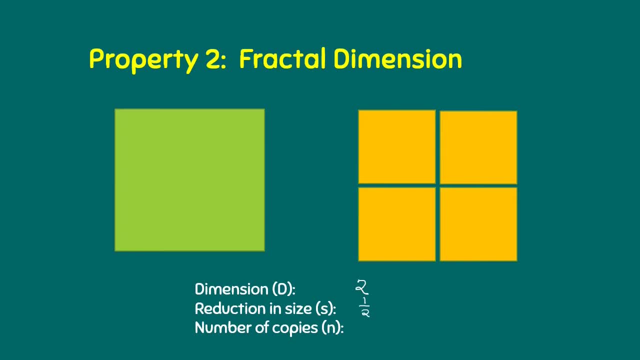 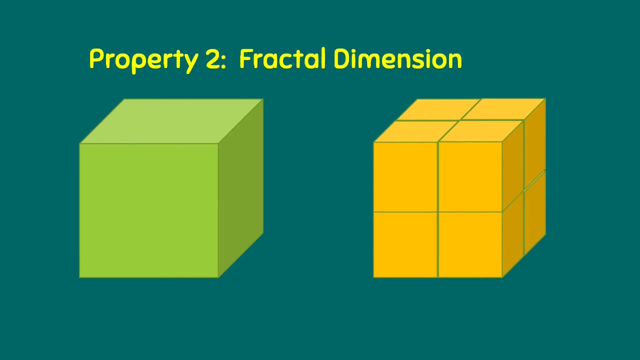 our triangle is still equal to one half the number of copies. we ended up with four smaller copies of the original square. next, let's look at a cube 3d, a three-dimensional object. so, similarly, just what we did in the previous slides: we also get the midpoints, we also get the midpoints and. 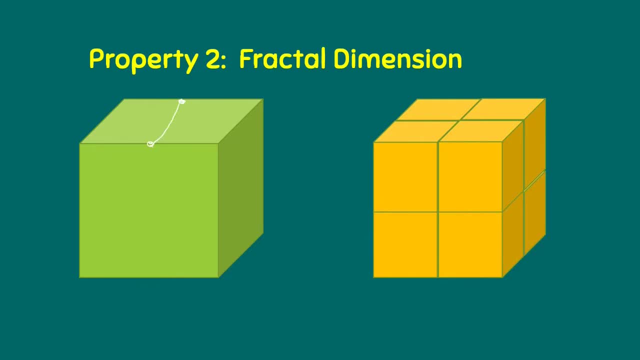 then we cut the cube along those midpoints. okay, so before we do bonePac characters, the finalhhhh. when we do that, we will end up with this pattern over here. so what happened here? so our dimension, our dimension is three: reduction in size against we are always looking at one half because we are always dividing the segments into two and 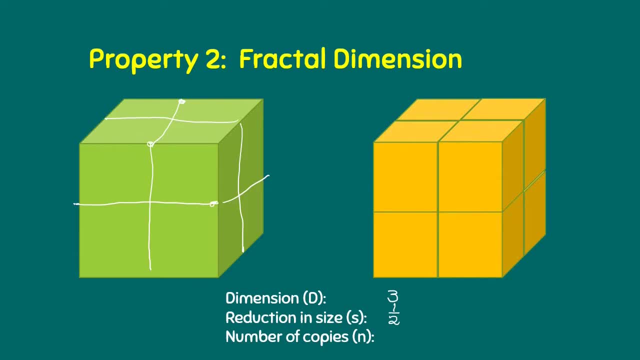 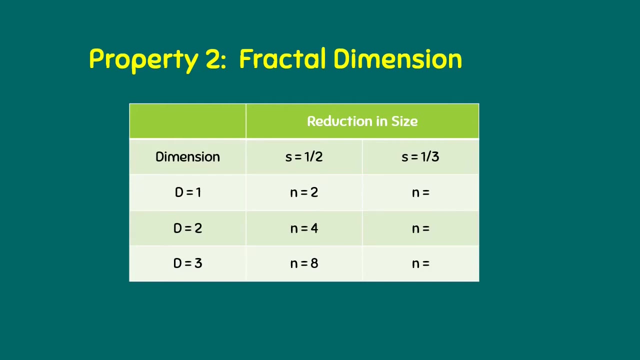 the number of copies. how many smaller copies of the original cube did we end up with? we end up with half of the same, just because of we keep dividing the brackets. local alyca was given to usubzęf. tayal ended up with with eight equal copies. okay, so here is a summary of um what we did so far. 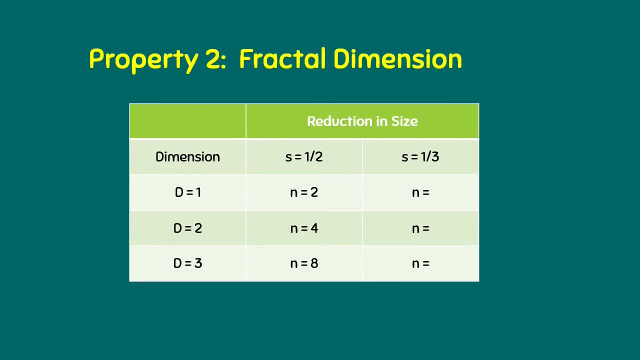 if we have s equals one half, if s equals one half, we had two copies. if d is equal to one, if d is equal to two, we ended up with four copies and then, if d is equal to three, we have eight copies. now what will happen if s is equal to one third? so, meaning to say we always divide the segments into: 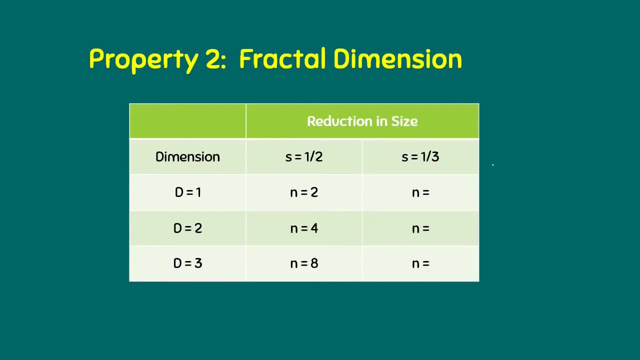 three equal parts. so, for example, we have a line, then we divide it into three equal parts. what will be the number of copies? so, of course, the answer is three. what about if dimension is two? so if we have a square, we divide it into three equal parts. the segments: we divide the segments. 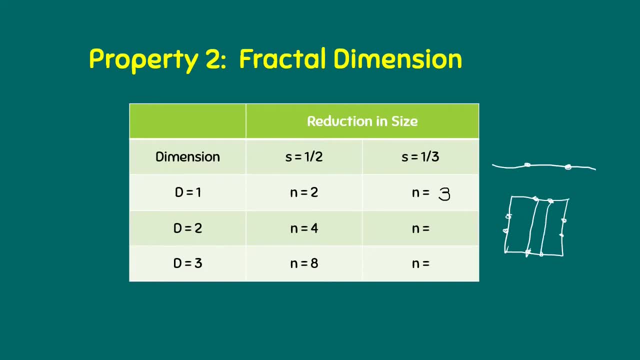 into three equal parts and we end up with three equal parts. so now what will happen? if s is equal, three equal parts. we end up with how many smaller skip, how many smaller squares? we end up with nine. can you guess what will be the number of copies if, uh, and is, if the dimension is three and s is 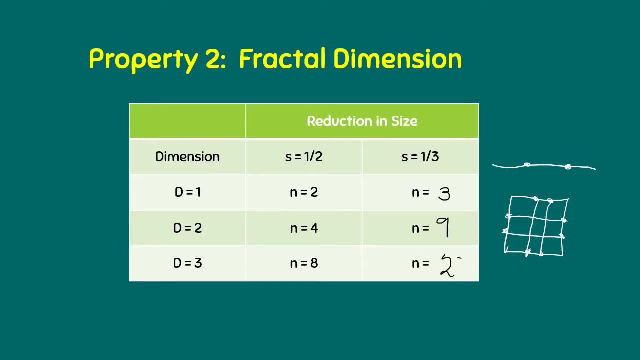 equal to one. third, the answer is equal to 27.. now, what is the pattern behind this number? so, for example, here, what is two? two is equal to two raised to one. so these are all powers of two, right, this is two raised to two. this is two raised to three. in this case, this is three raised to one. 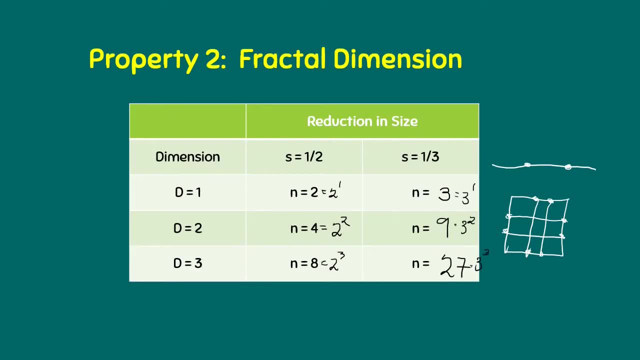 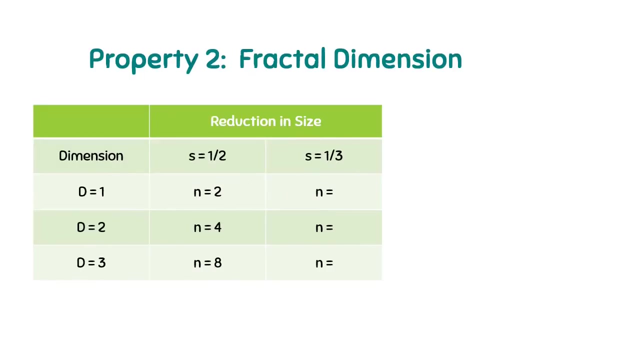 this is three raised to two and, lastly, this is three raised to q. so, if we try to generalize that, what can be a general? what is now the relationship between d, the mentioned s, the call it, the magnification factor, and um n, the number of copy? okay, so here is again. 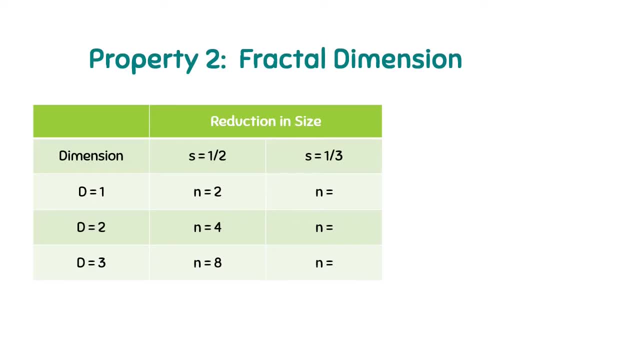 out the table that we obtained. um. let us now try to decipher. what is the relationship between the values d, s and n? what do you think? the answer is this one: the number of copies is equal to the reciprocal of s, correct, um, remember, recall that. okay, here, this is three, three, three, three. 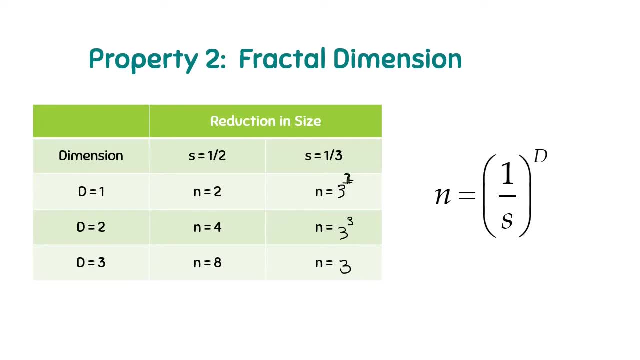 squared three, q, uh sorry, three raised to one, three leads to two and three days to three. so the base here is always equal to three, and that is the reciprocal of s, correct. similarly, with this one, the base here is always equal to two, correct, and two here is the reciprocal of s. so therefore n is equal to one over s. 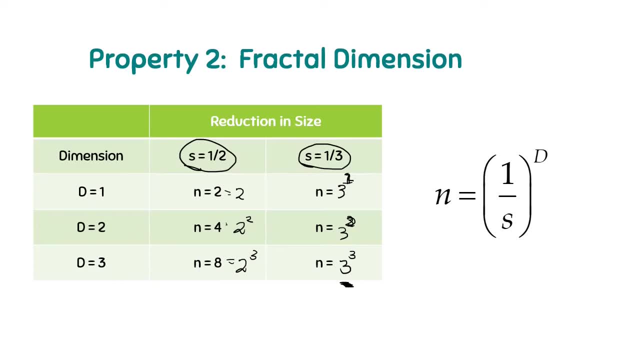 raised to d, but remember that d here is the d, here is the dimension. so therefore, we want to solve for d. so, if, if, from your algebra, how do you solve for d? if he appears as an exponent? we take the logarithm, both sides correct, In order for us to bring down the exponent. correct, Because from the 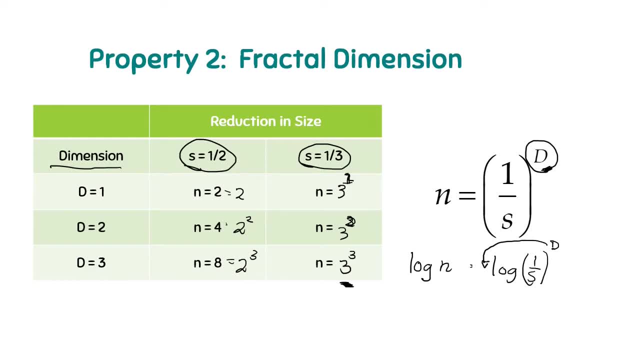 properties of logarithm, this exponent over here will go down, So we have d. log of 1 over s is equal to log n. So therefore, since we're solving for d, we divide both sides by log of 1 over s. So that's it. Therefore, our d is equal to. 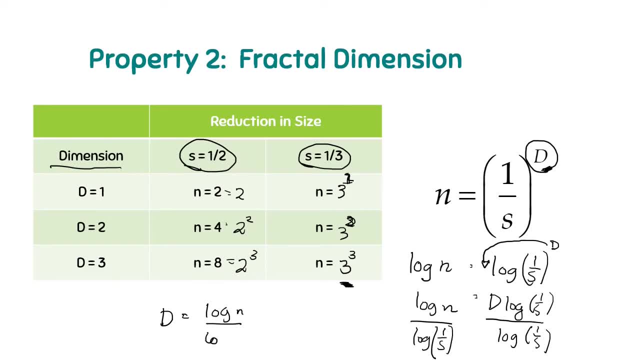 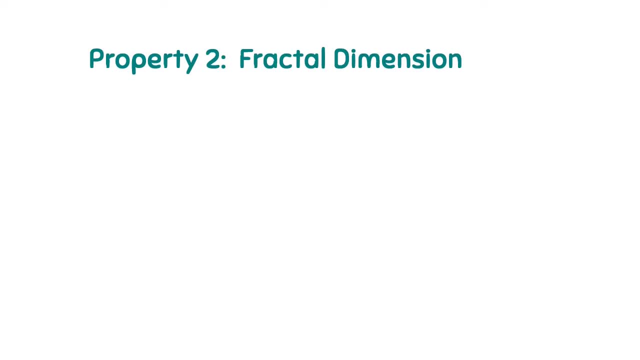 log of n over log of 1 over s. Okay, let me just write here the. what's this? the formula that we had for d, We have d is equal to log of n over log of 1 over s. Now n here is the number of copies, So that it: 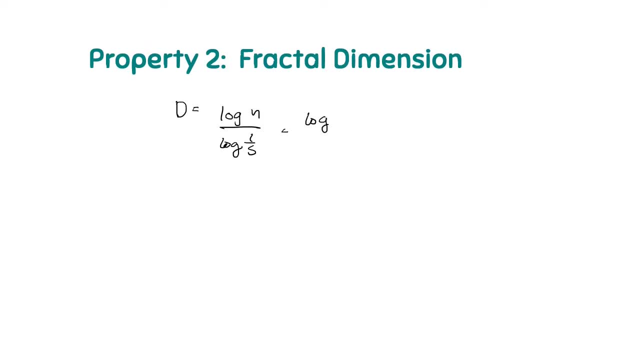 will be easy for you to remember. You have to know what the variable stands for. So n is the number of copies, And 1 over s. here is our magnification factor. Okay, so remember that. Now, what can we say about this? 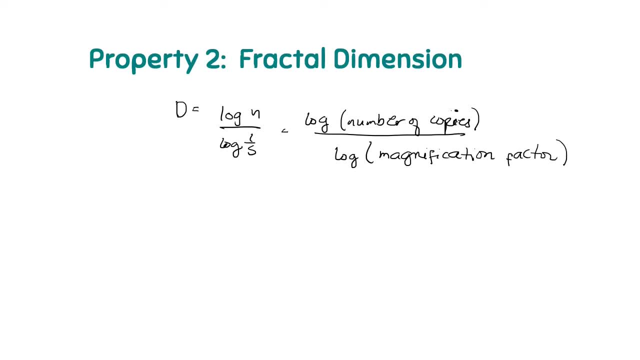 this d over here. Now take note that this number is not a whole number, correct? So that's. so. it's a fraction, right? So that's why I. that's why where the, the uh scientist um got the. 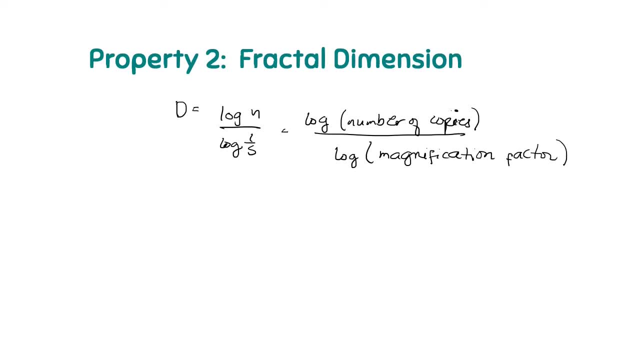 the name for fractals. They named it fractals because um, it is a fraction, Although it's not a rational number. ha, It's an irrational number, Although it can be expressed as a fraction, but it cannot be expressed as a fraction where in the numerator and denominator are whole numbers. 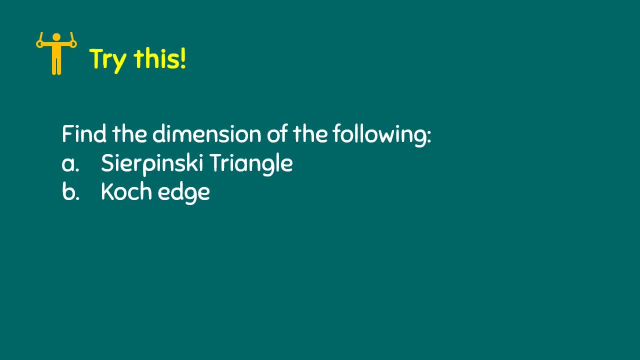 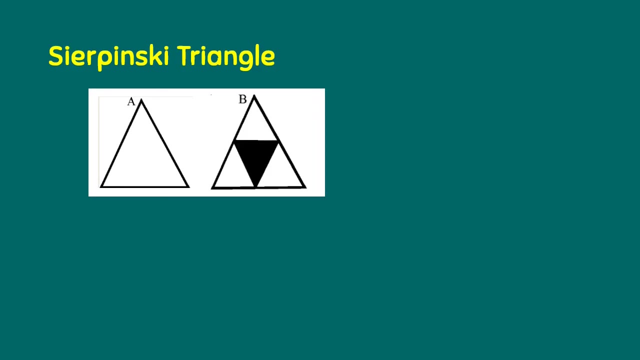 Okay, so let's have a few exercises. What we want to do is to find the dimension of the following: Sierpinski triangle and Koch n. Let's start with uh, Sierpinski triangle, um here, But we have to get our n and s. Okay, what will be our n here? 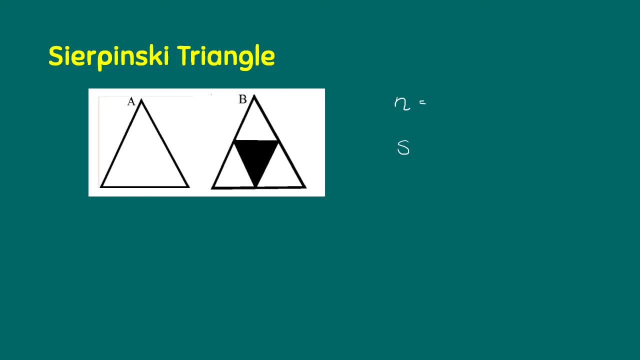 So we started with a white triangle and we ended up with three smaller white triangles, right, So our n is three. What is our s? Our s here is equal to one half, correct, Because, remember, when we constructed the Sierpinski triangle, we divided each of the segments into two equal parts. 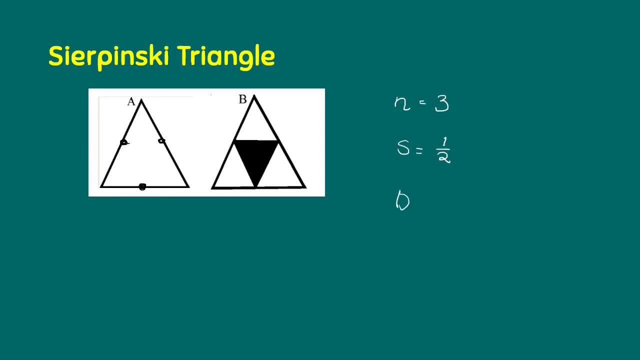 So using our formula d is equal to: let me just write that log n, log 1 over s. So this is log of 3 over s, Log of 2. And that's approximately equal to 1.58.. 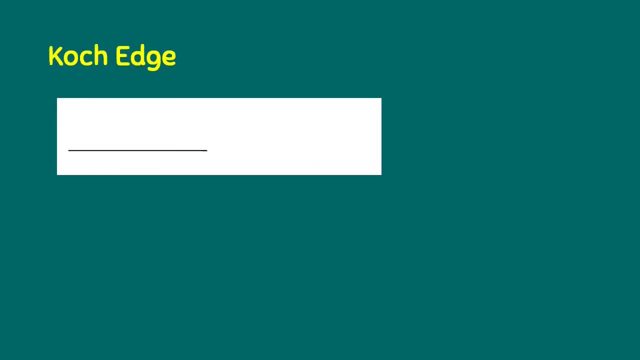 Okay, for the Koch edge, we have a segment and then we divided it into three equal parts, right. So therefore, our n and what we need and n s, Our s is one third, correct, Because we divided it into three equal parts. 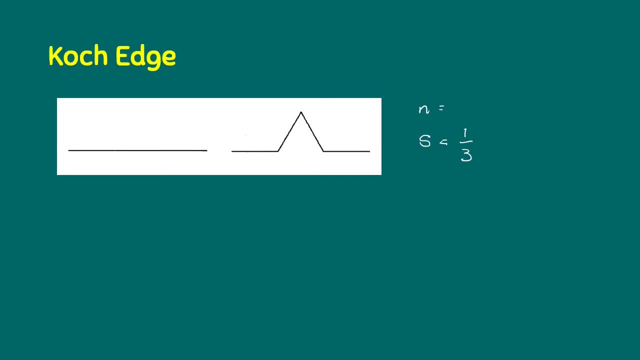 And then our n, we ended up with four copies of the original segment, correct? So therefore, what is the dimension? d is equal to log of the number of copies, which is 4 over log of 3. And that's approximately equal to. 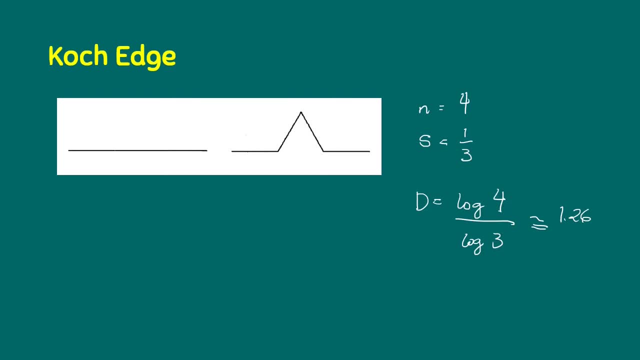 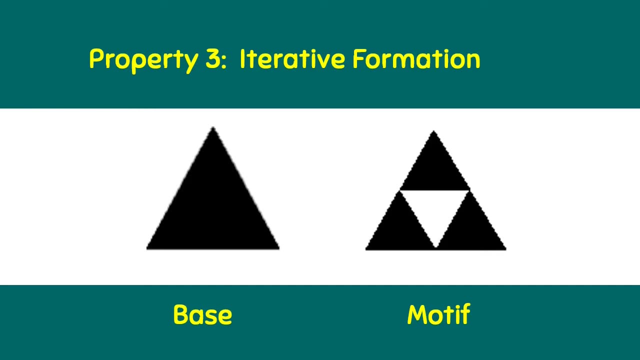 1.26, okay. Next property of fractals is that we have already seen this before- that they have iterative formation, Meaning to say we can get the fractal simply if we know the base and our motif. So, for example, in our Sierpinski triangle, this is our base. 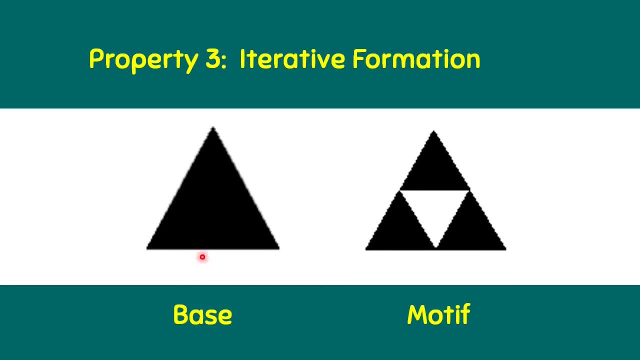 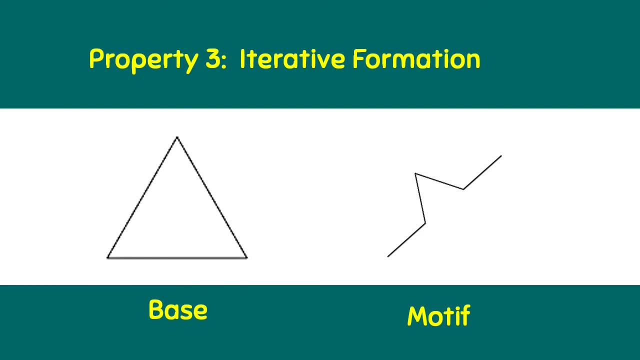 And then, if we already know that this is the motif, meaning to say that you already know that the pattern is This one. Every time you get a black triangle, you repeat this process. You always have a base and a motif. Now, for example, this one is a Koch snowflake. alright, 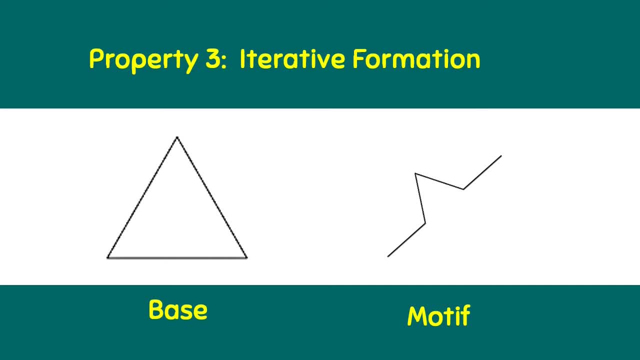 So what happens here is the difference between a Koch snowflake and a Koch edge. For a Koch edge, we started with just a line segment, right. However, for a Koch snowflake, the base is our triangle. And then what is the meaning of this part? that the motif is this: 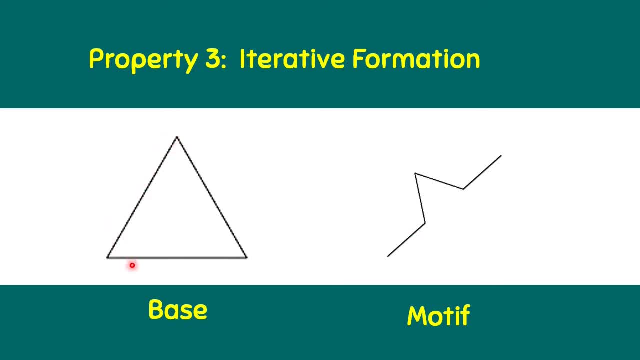 So every time you see a segment here, you always make like a version of a Koch edge here. So it's like a Koch edge, right? And then three of those, alright, Put them all together, Okay, Okay. next we want to construct the dragon curve. 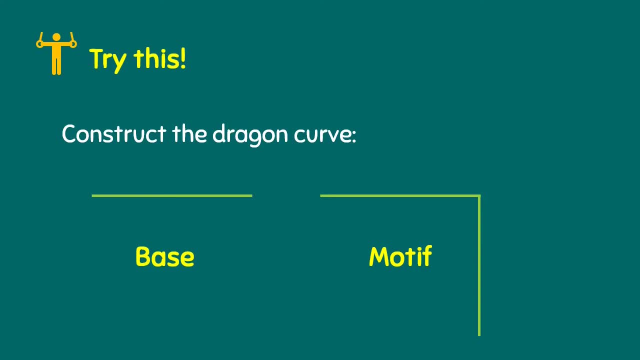 So we have a base, This one. we start with a line segment, okay, And then what happened here in the motif? So this one, you copy it, and then you do it, you copy it and attach it to itself by 90 degrees, correct? 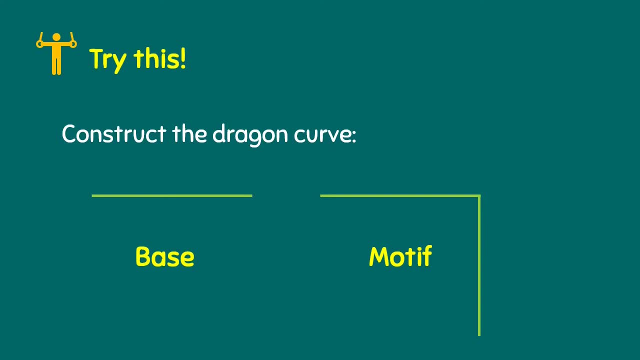 Okay. So how will we now construct the, The dragon curve? So here is what we are going to do. Let's just try this for the first. Okay, let's continue this one after. This is the. Let's iterate this process. 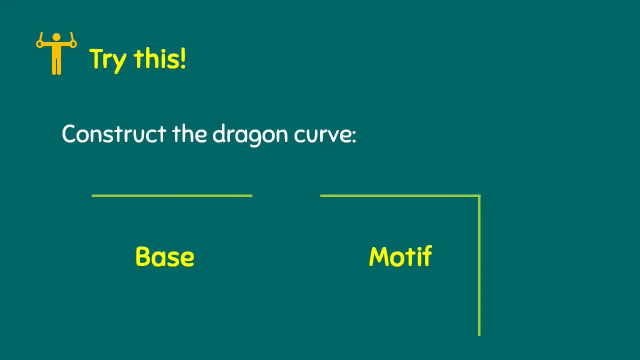 So meaning to say we copy this right, And then we make a copy of this, and then we attach it to itself by 90 degrees, And then we attach it to itself by 90 degrees, And then we make a copy of this and then we attach it to itself by 90 degrees. 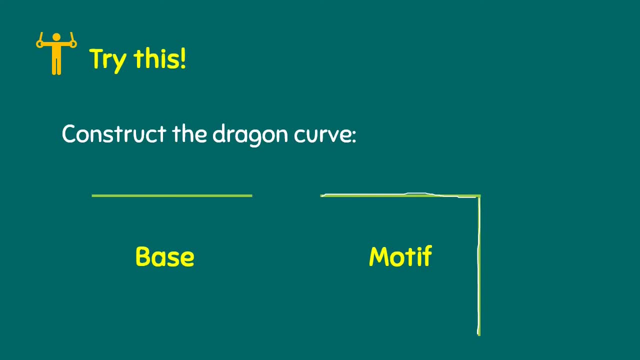 And then we attach it to itself by 90 degrees, And then we attach it to itself by 90 degrees. All right, So how will it look like? All right, So how will it look like? Okay, so I have here the original figure that the- I mean the motif that we have, and then I just turned it smaller. 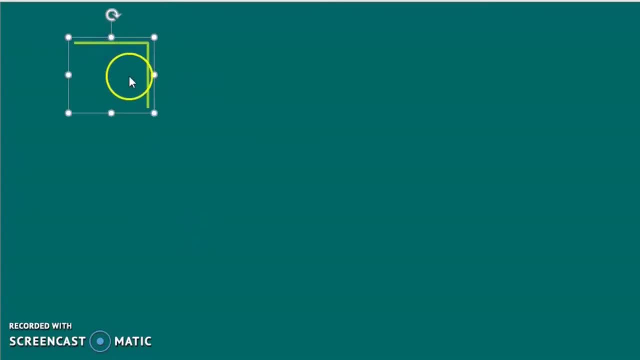 Okay. so what will we do? Okay, so what will we do? We copy it Okay. control c, control v. copy it right, Just so that you can see that. okay, Just so that you can see that okay. 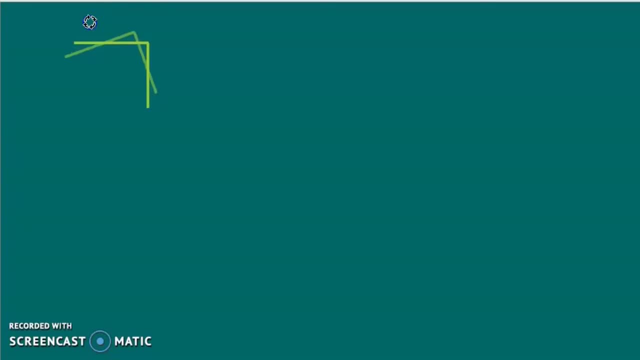 That's it, And then We just rotate it, oh, And then We just rotate it, oh, But it should be around 90 degrees. But it should be around 90 degrees. that point correct. but when I'm rotating I want it in such a way that the point 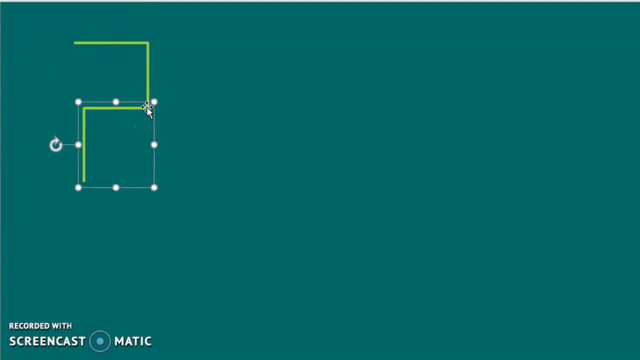 it was originally here, right, okay, and then next V, again copy, and then control, and then let me just group this thing, alright, and then we will. maybe I should, I should just make space, okay. so this is remember the second copy, alright, and then I will attach it to itself because it's moving. there you go, and then 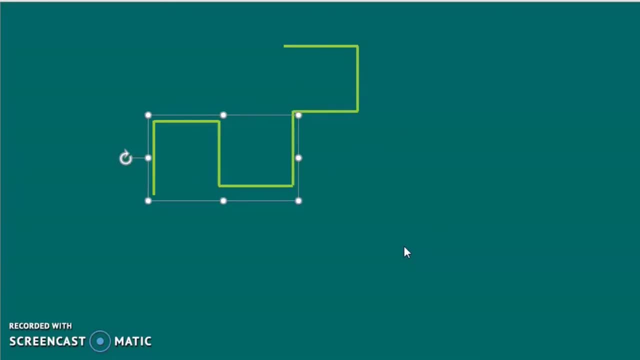 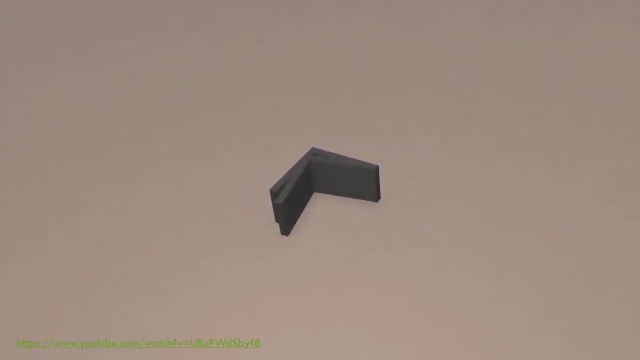 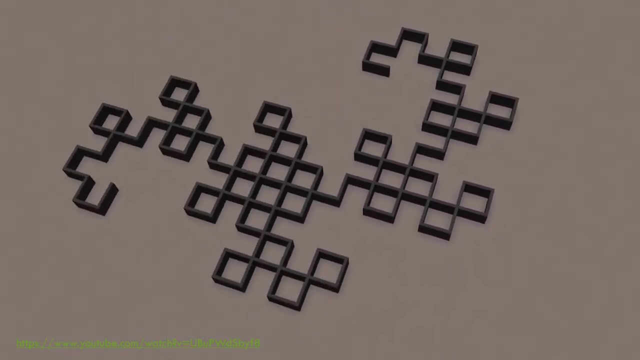 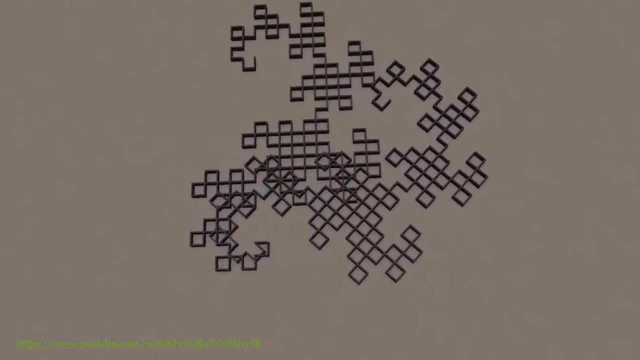 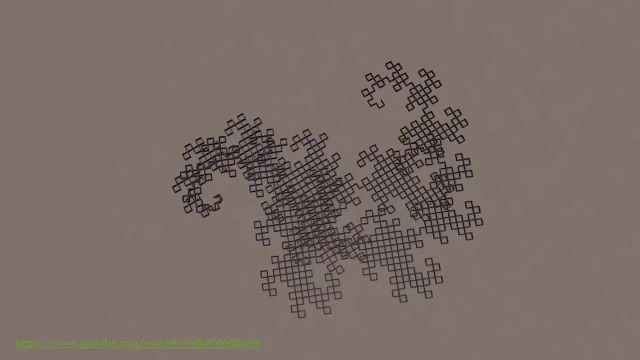 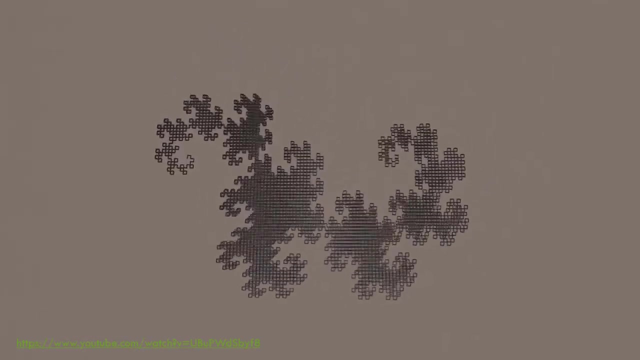 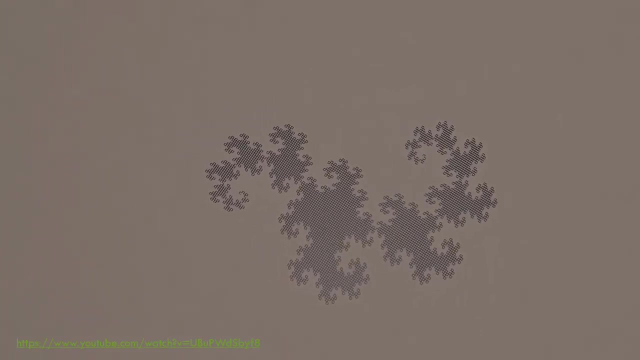 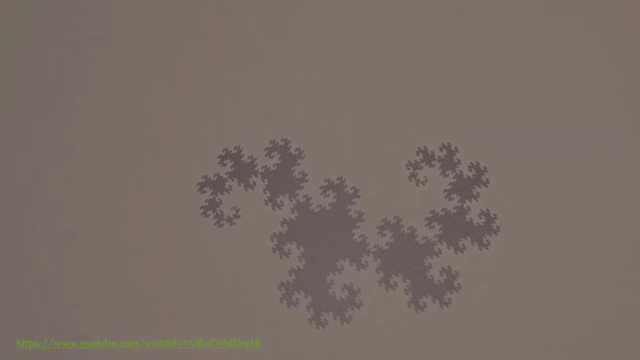 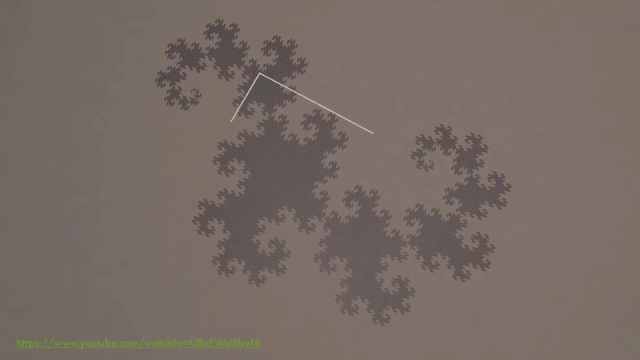 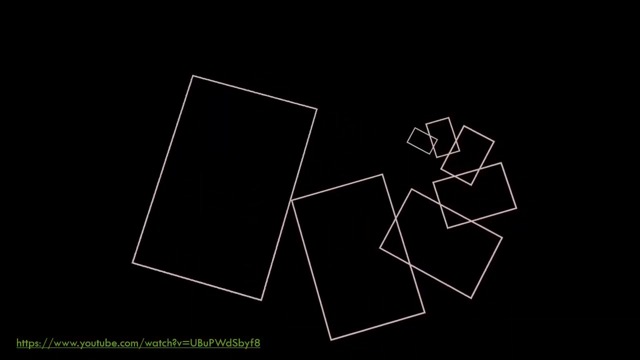 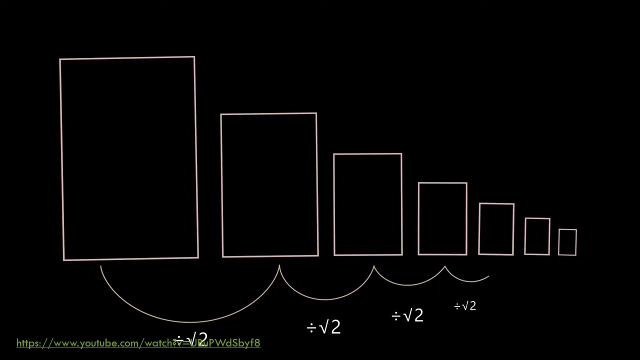 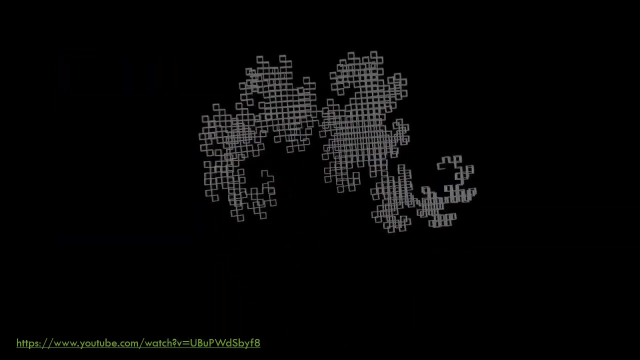 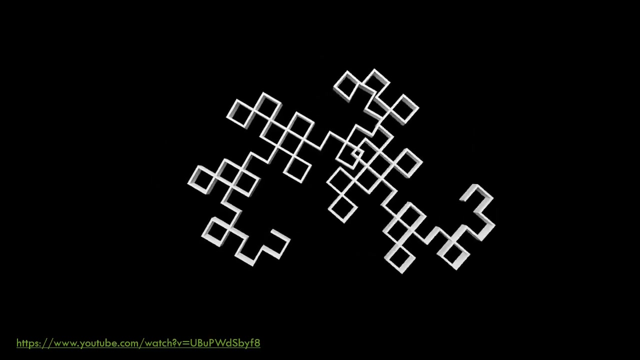 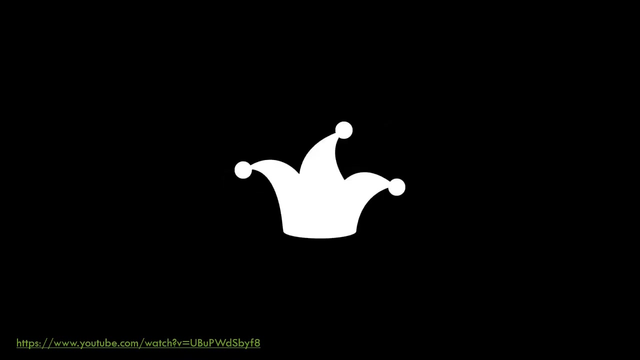 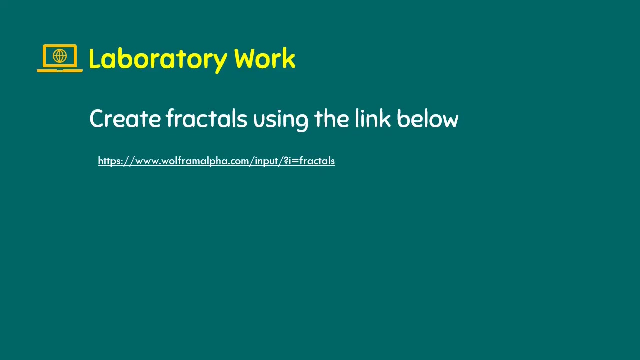 you will continue the same process over and over again so that you can see how does this iteration really works? um, let us watch this next video. so, you, you, okay, so we can actually make uh, uh uh fractals using um this uh link wall from alpha. let's just go to that one. 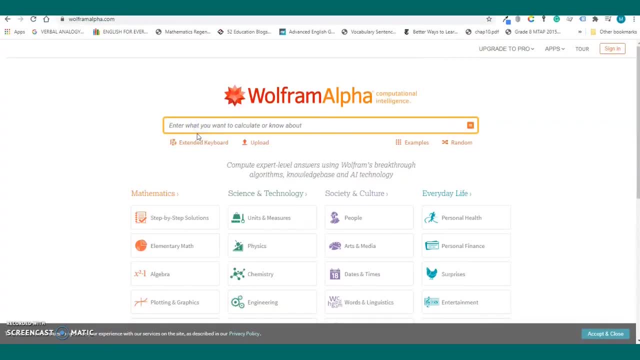 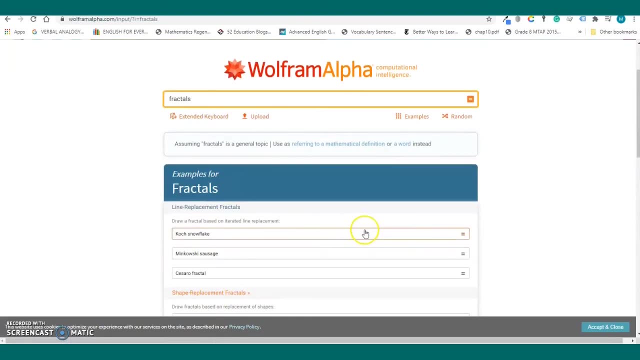 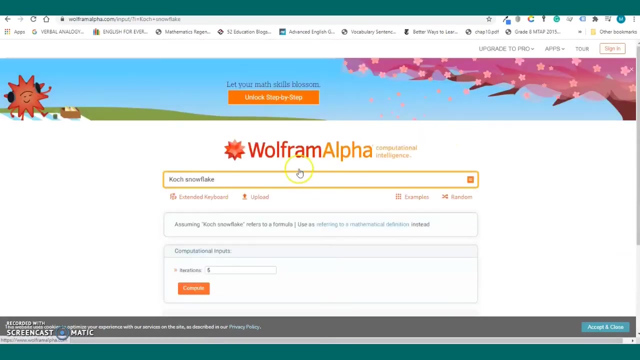 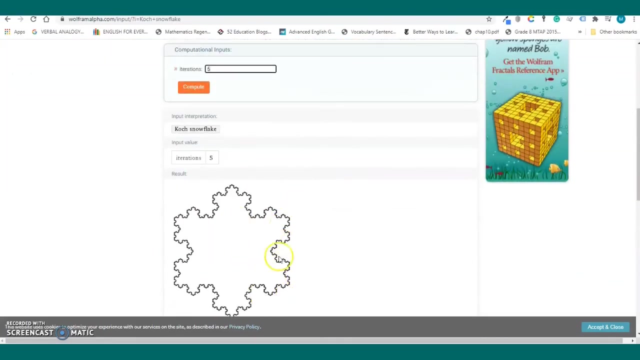 all right, so you can just, you can just go to wallfromalphacom and then you can just type fractals, and then here are the factors that you can make. so let's just see the first one. so the maximum here, because this is not paid version- the maximum iteration that you can make is five. okay, so you can make. 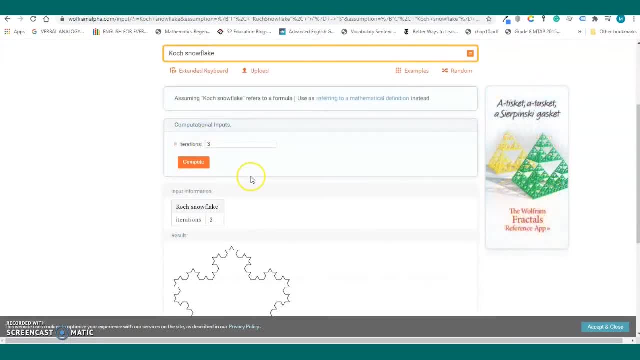 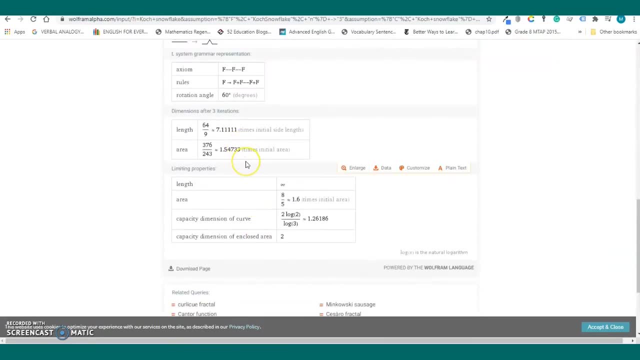 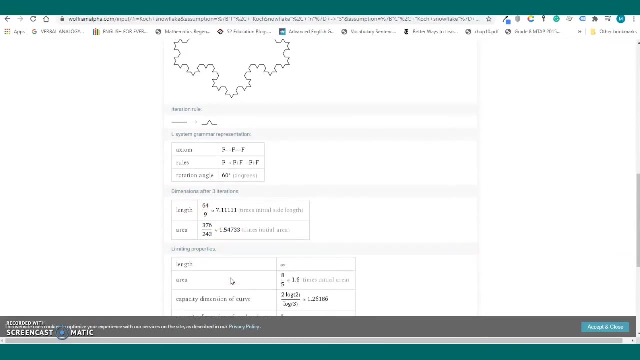 it smaller if you want, so for example, three. so this is the coke snowflake, that, um, you can get all right. so you have here the, the dimension also, okay, and uh, uh, the dimensions. after three iterations, so it can give you the length, the total length and the. 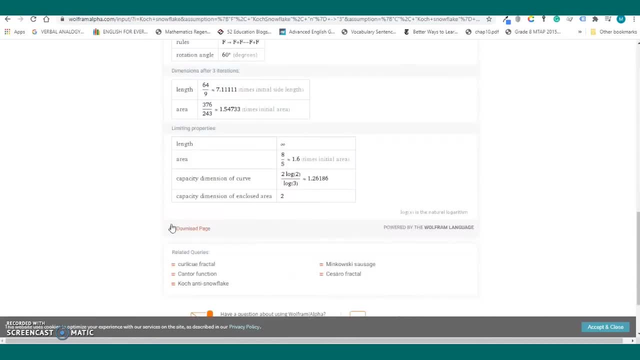 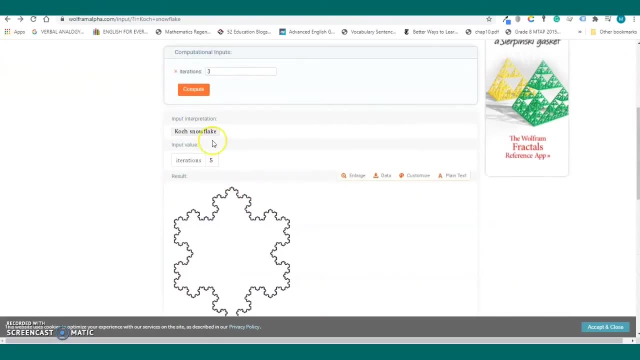 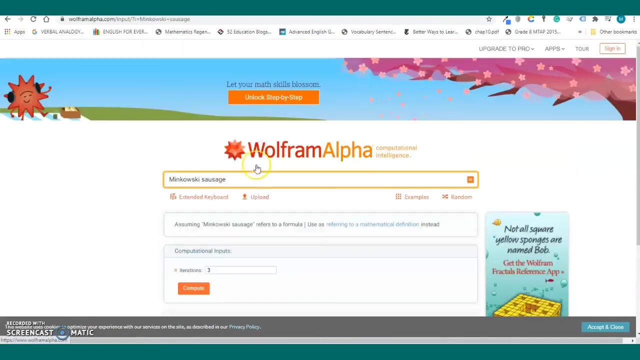 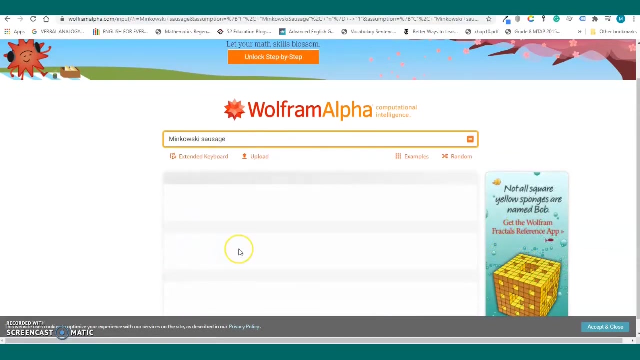 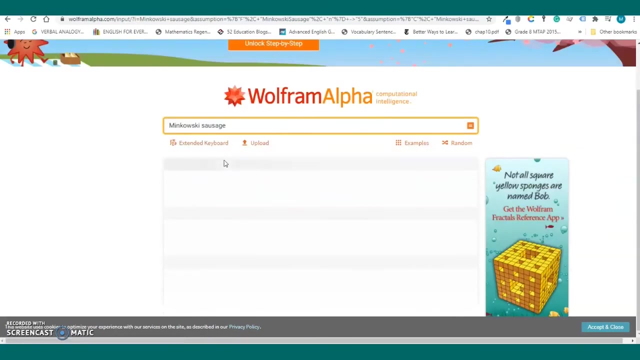 uh, area, okay, what else? um, let's go back, let's see what, what, um, what factors you can also. what is this? the minkowski sausage. so let's just make it one iteration: the minkowski sausage. if you have five iterations, the maximum, okay, so this one, all right. okay, so this is. 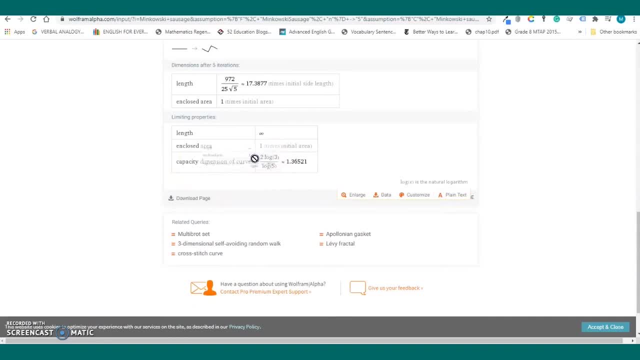 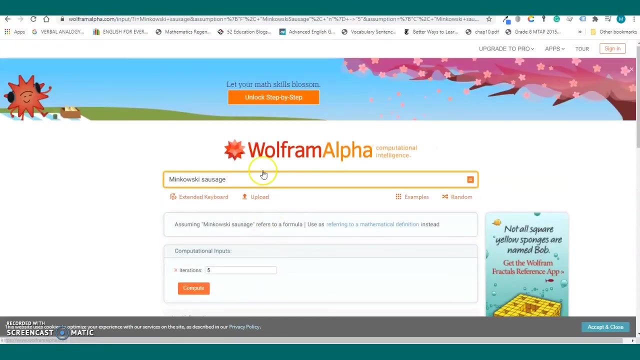 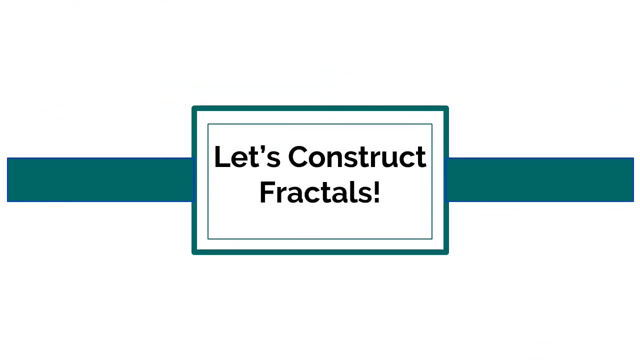 it's also giving you the the dimension. this is the, this is the um. what's this? the formula that we had earlier? all right, so there are many different factors that you can um get from this website. okay, okay, let's construct fractals. so it's just like what we did earlier. so what is the next figure here? 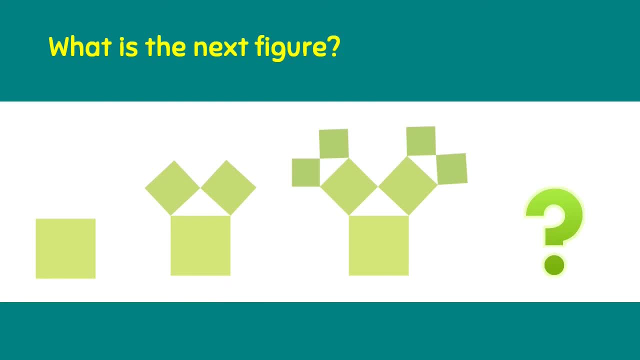 um, you can see here, this is the base and this is the motive, right? so what happens is that? what is the pattern here? um, you're getting two copies of itself right, and then you put them on top right and then, um, at 45 degree angles in each other. so what happened? there is this one you get. 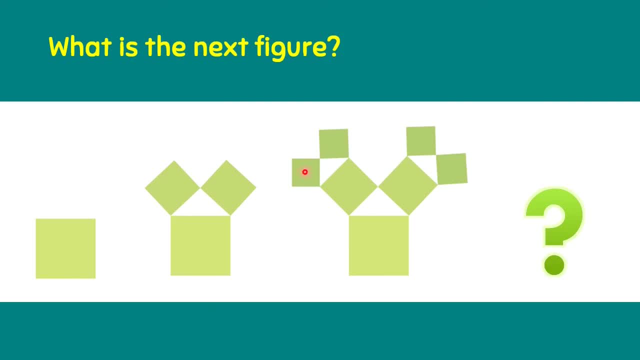 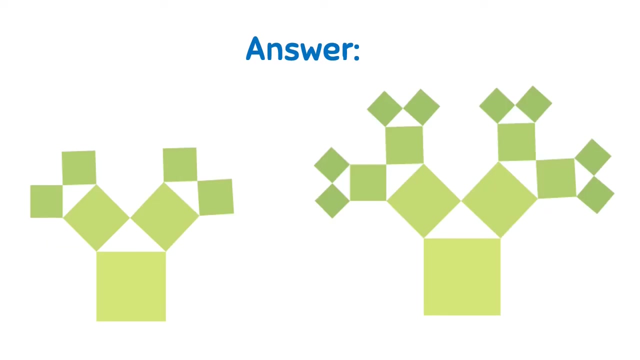 two. so for the next pattern, you get two smaller squares again and then put it on top. put it on top- okay. and then similarly again from here you get two smaller versions of itself, correct, okay, and you will end up with this one. so this is the last figure that we had. 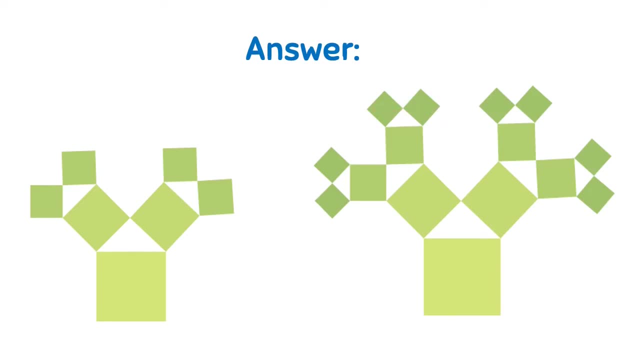 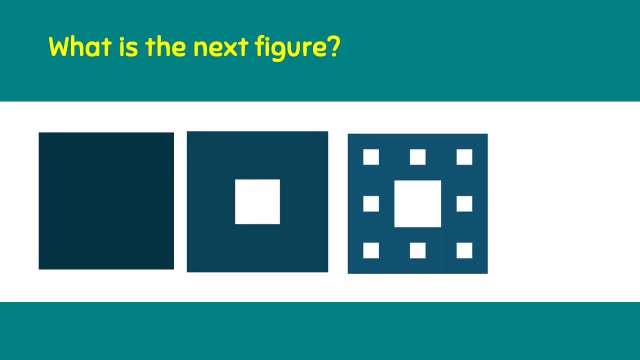 okay, and then these are the two. right, these are the two. this is what the squares that we added on this isolation next, um, what is happening here? what is the pattern here? what's happening is that. this is the pattern here. what is happening here? what's happening is that. 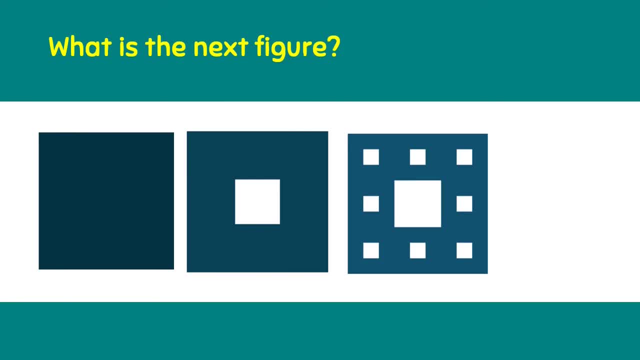 so, basically, how did we divide the segments? so, basically, how did we divide the segments? what, although you may not see it here, what, although you may not see it here: the original square. you divide it into the original square. you divide it into any equal parts, right, and then connect. 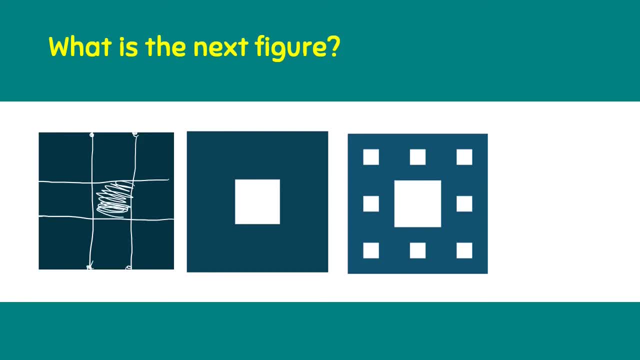 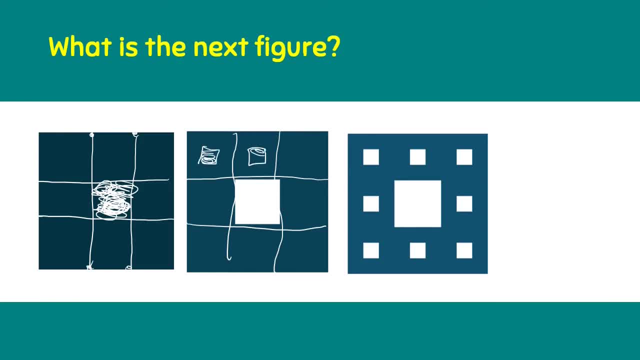 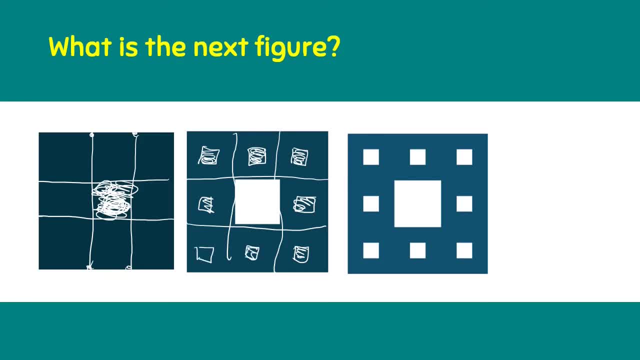 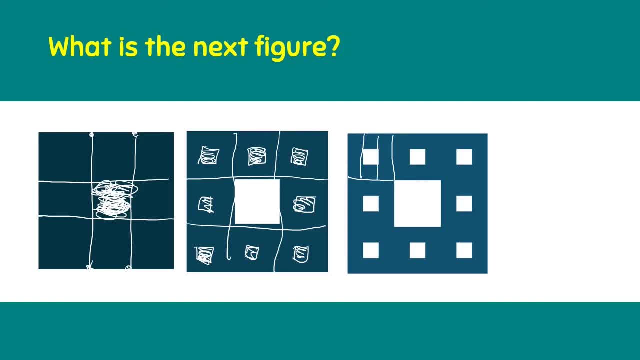 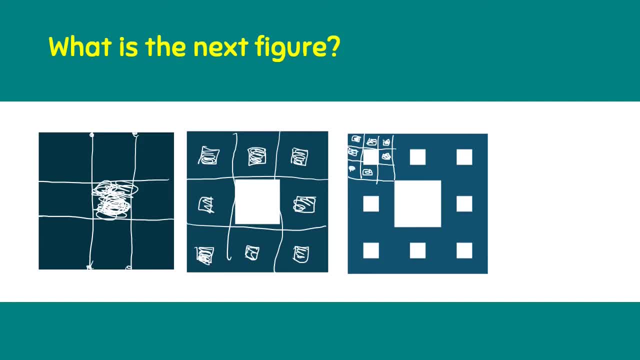 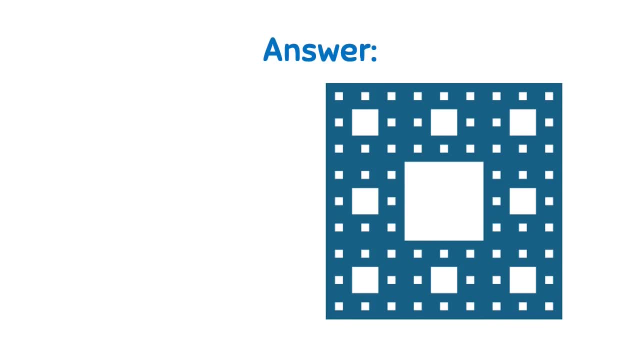 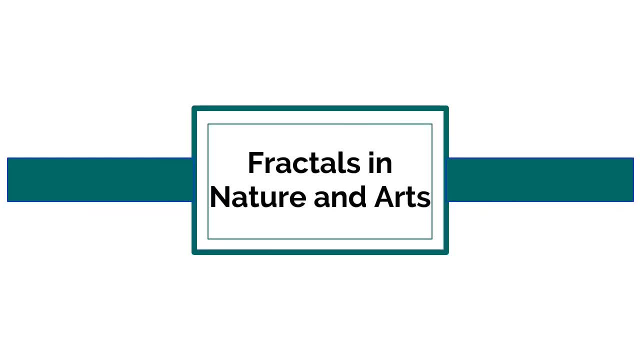 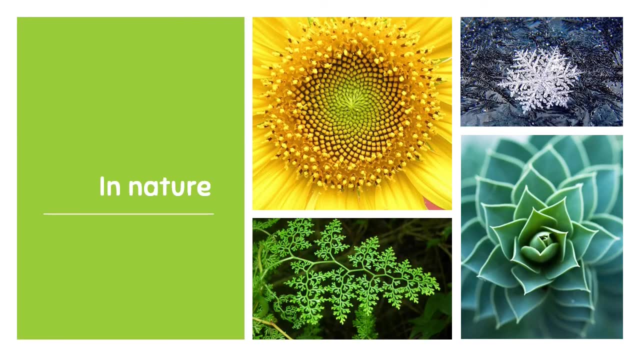 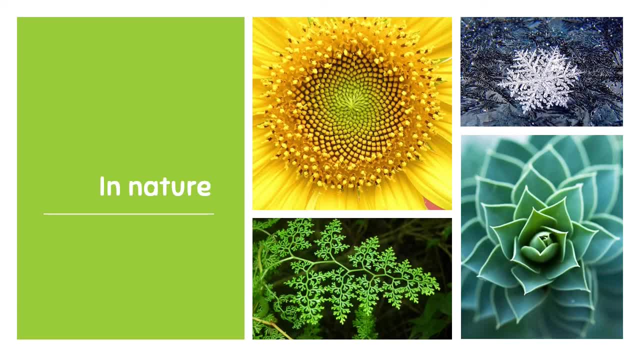 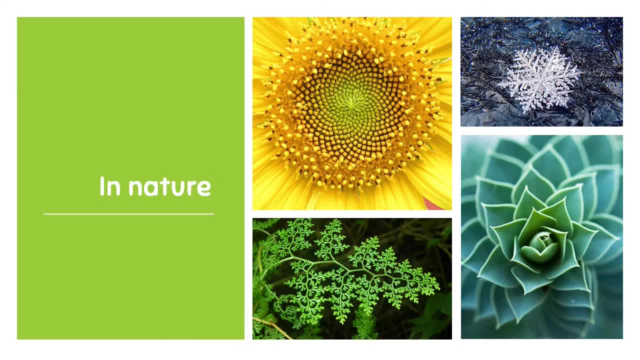 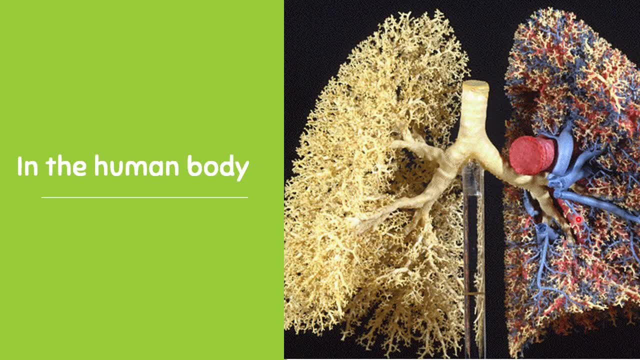 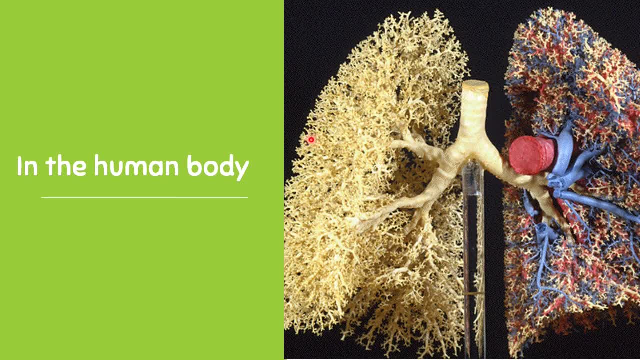 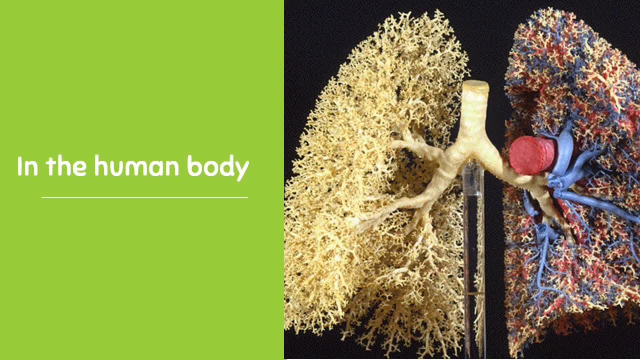 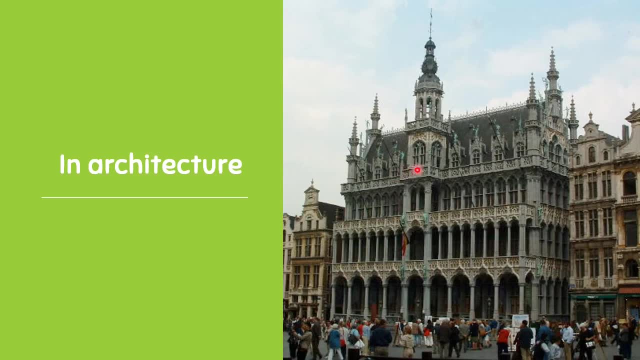 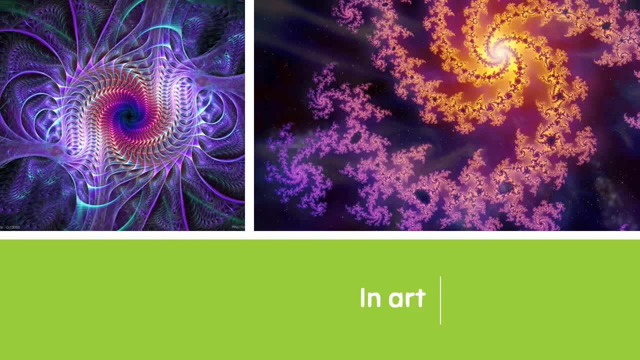